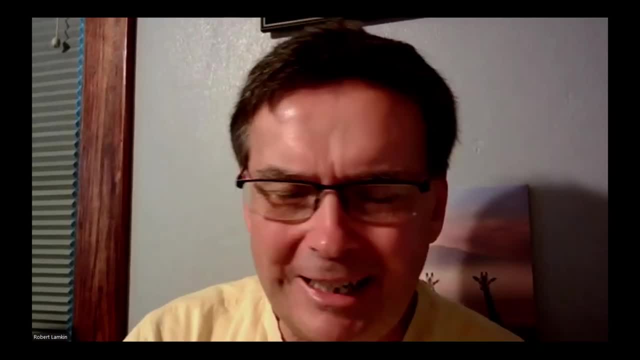 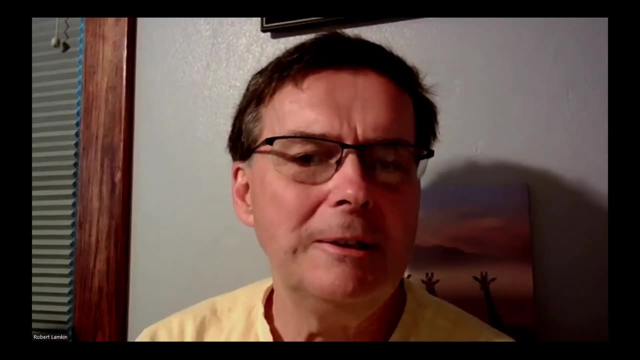 And it's like: oh man, what you know, I didn't get this, I want to. I wanted to get that too, And- and this is kind of the way it is for me, you know putting together these lessons, and especially with areas, regions like this, 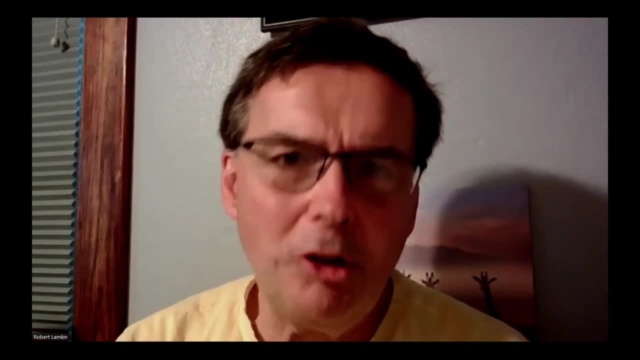 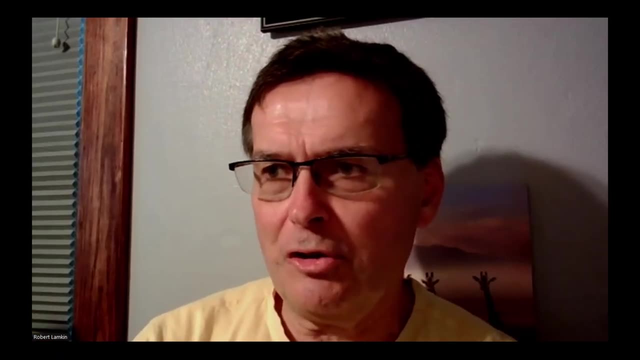 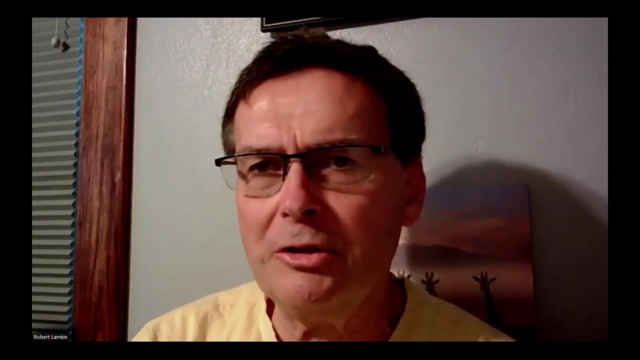 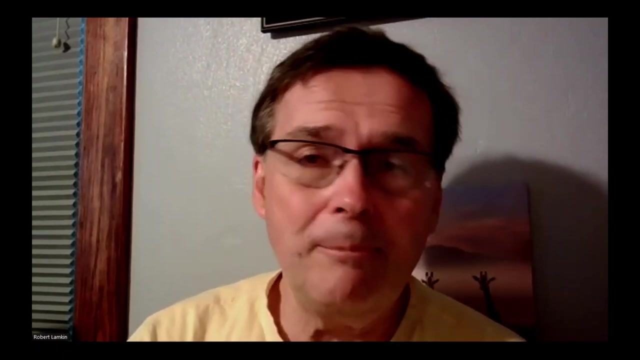 And, like you know, I just I wanted to. I really want to cover China's belt And the road initiative it encompasses. so much in regard to the nervousness of the US, China's neighbors and maybe increasingly, other areas of you know what's China? you know China. it seems to be getting their nose into a lot of areas around the globe via infrastructure. 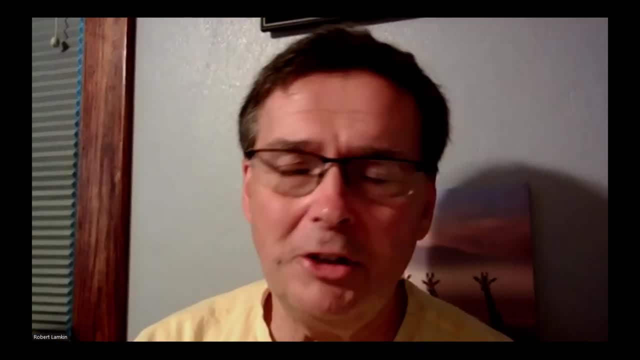 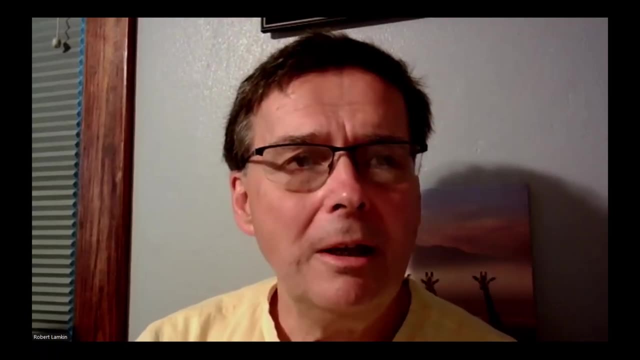 And I don't have time to develop that right now. It's in your textbook And I'm not going to cover it with the lecture, but I didn't know what to cut. you know, And as I say that I may, but you know I'm taping this during the summer months. 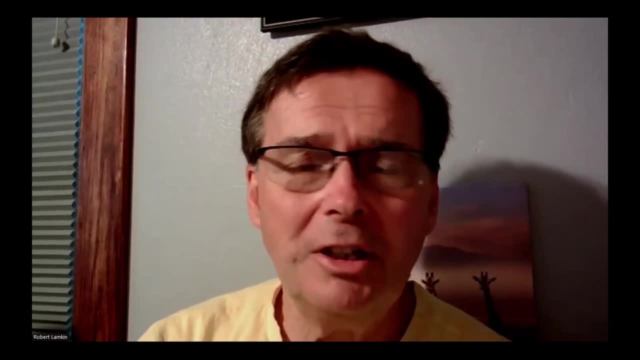 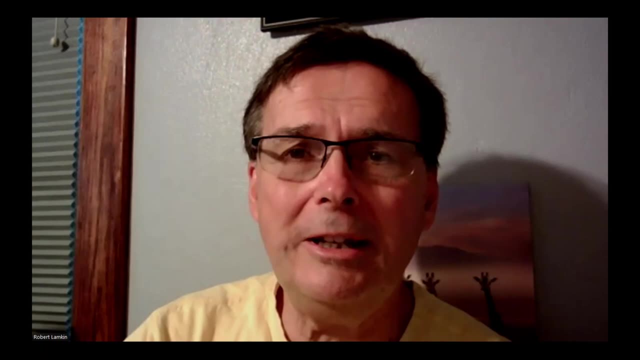 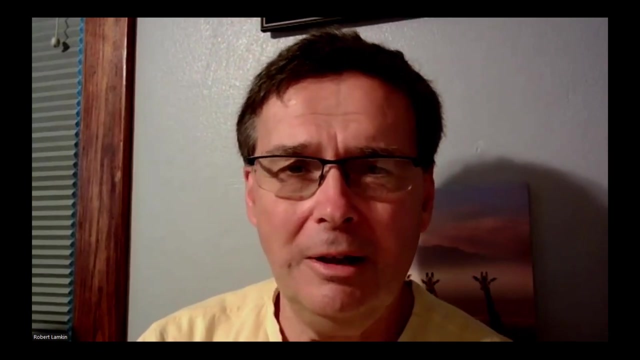 By the time we get to this, there may be a announcement for you guys that we are. I'm going to have you read this section and there will be quiz questions on it. As I sit here at this juncture, I'm not doing that. 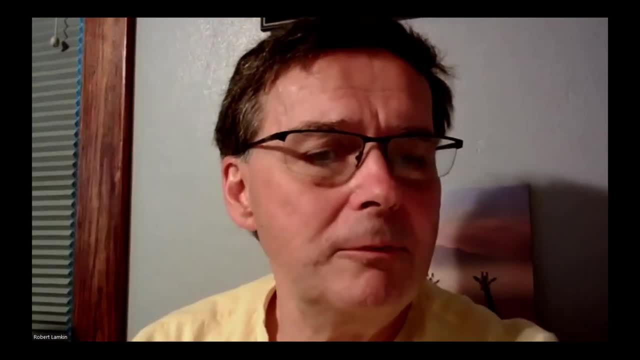 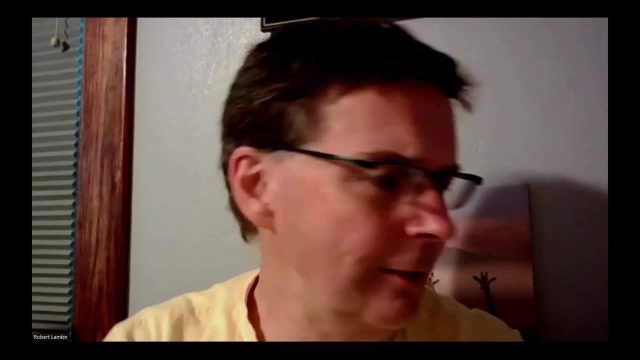 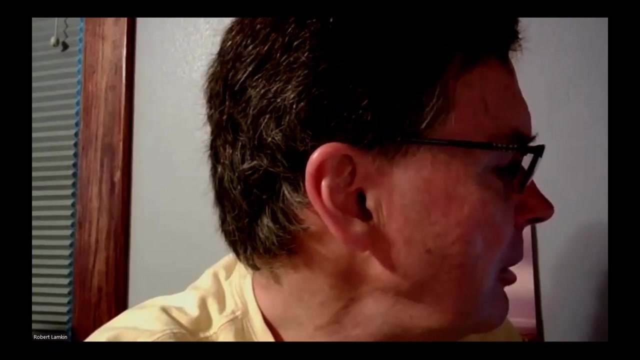 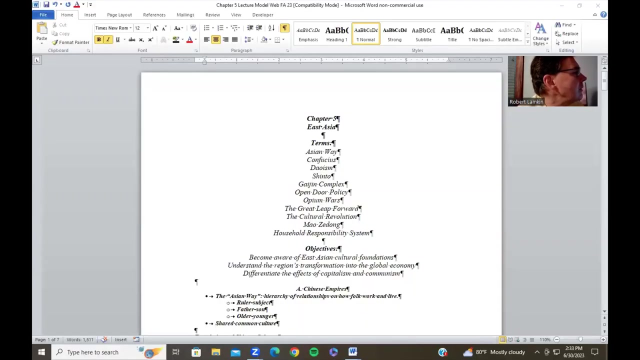 If you have your textbooks, you should by now your visuals. you can turn the page to 275. And as you're doing that, I'll do what I like to do and get the screen share up. I do not want that. 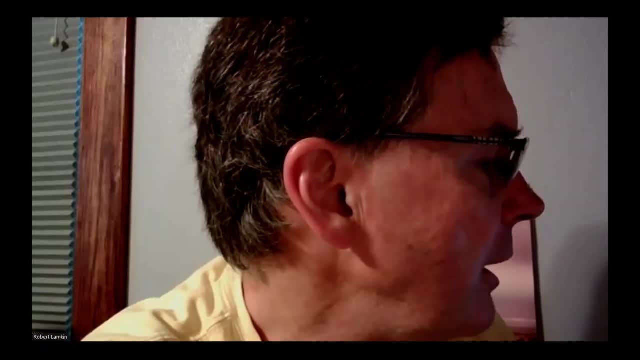 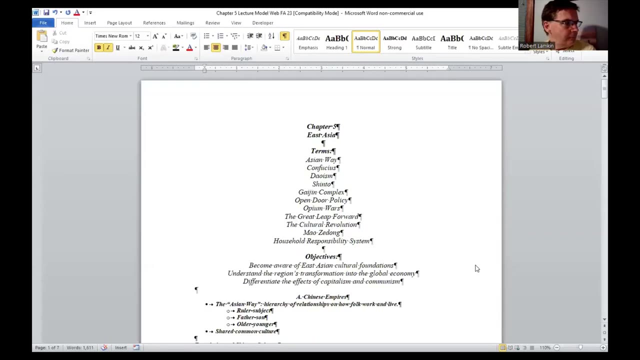 Okay, Hit the wrong button here. I apologize for that. Let's try that again. This is what I want, Okay, Yes, East Asia. Some of the Got that backwards again and should get the objectives up there first. I like to talk about that. 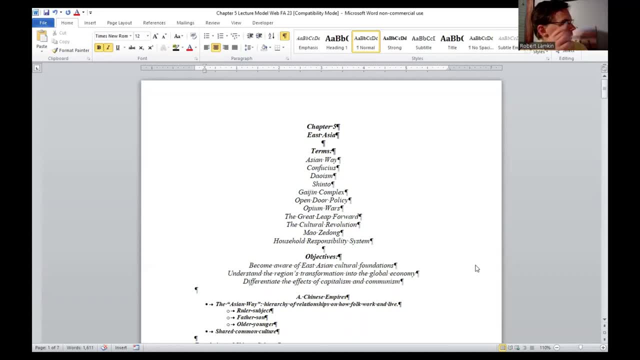 I guess it doesn't matter, I just like my routines. Objectives: We want to become aware of East Asian cultural foundations, Understand The region's transformation into the global economy and differentiate the effects of capitalism and communism. All right, Major heads up terms here. 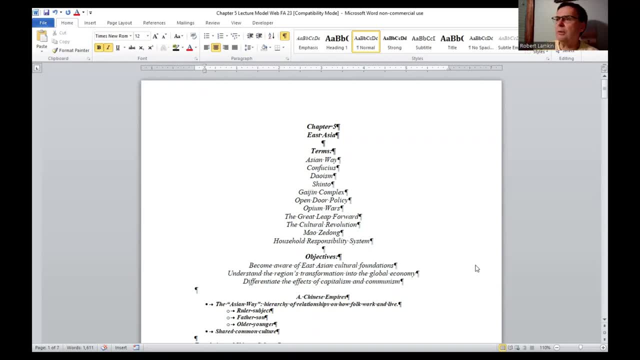 The Asian way, the Asian way throughout the region. There's a way that you're expected to relate to order, Um relational aspects of order, The way that you're actually entitled to the announcements of certain things and the exact people and the conditions that you should be looking for. 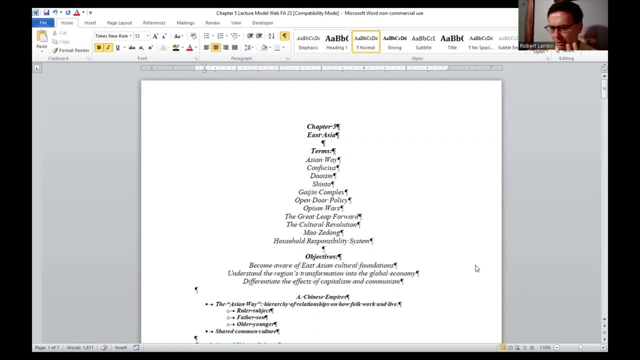 Well, the the thing about Confucius in a mode of finance. I think we don't feel like a lot of people have understood that, And so that's why I was coming in on my very first talk and I was talking about it. 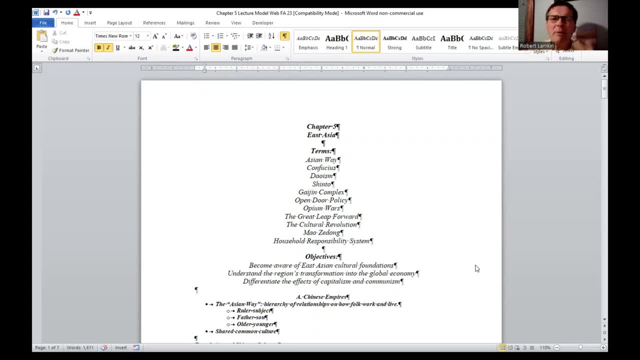 I've been invited by the Dalai Lama yesterday and- and I was talking about, um, you know, Taipei. I've been talking about it a lot And I always think that we have to really, You know, we have to really be rational with our ideas of what's going on. 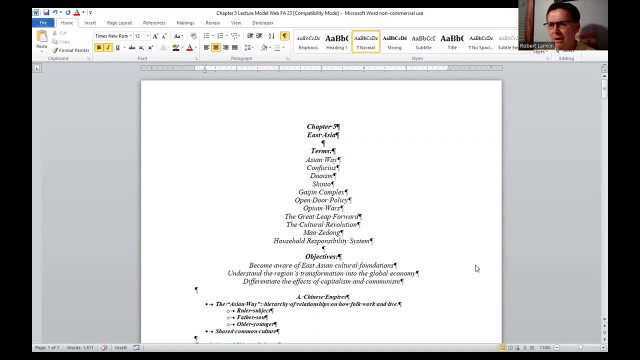 Uh, so we kind of have that common sense. If we don't, if we don't feel that way, then we're going to lose a lot. right with uh, one another, uh, confucianism order, uh, and you, uh, maintain that order by your. 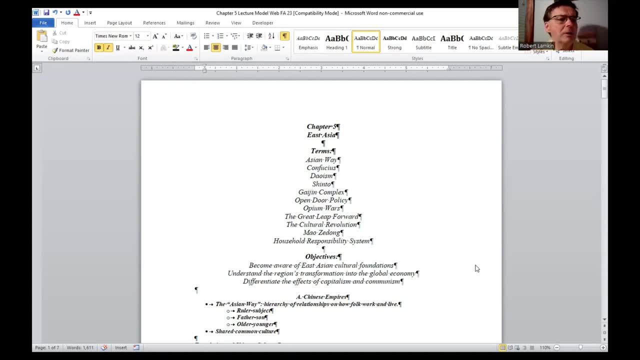 authority structures like the government. taoism it's more or less uh looking at uh. you know the universal uh goal, but the goal is balance uh between uh humans and the uh principles of the universe. right, shinto. shinto, the national religion of japan, the national religion of. 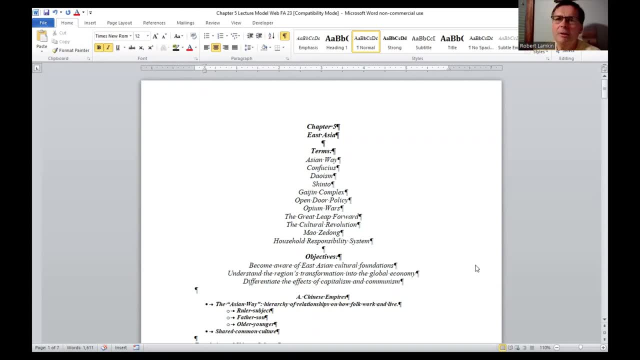 japan. we have, uh, we're, the gaijin complex. the gaijin complex, um, arguably, you know, we use the word racism arguably, um, maybe irresponsibly, uh, we use it to. you know, get what we want politically out of things. and, um, if you could, if you really wanted to take a look at maybe the, the um according. 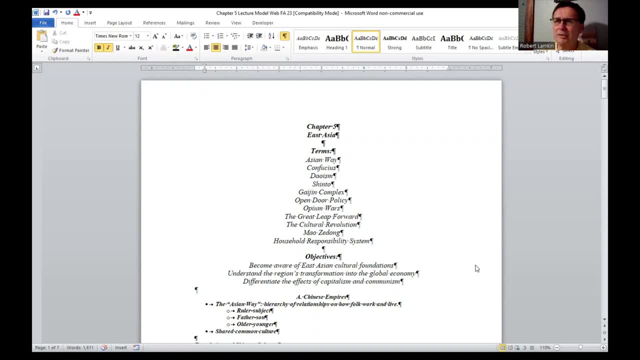 to the um correct vocabulary of racism, of feeling superior to another race. um might be a, a culture we're going to take a talk about today, and it's called the gaijin complex. uh, the open door policy. this is china opening up, opening up trade with the uh. 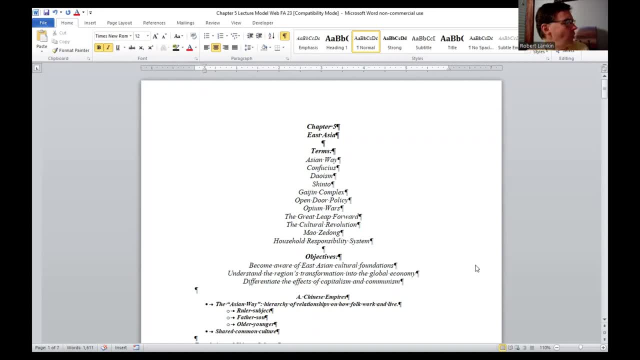 the the rest of the globe. the great leap forward, uh, great leap forward. uh just an atrocity on humanity. right mismanagement uh. in china in the late 1950s, early 1960s, 25, 30 million people die. uh. the cultural revolution: uh as bad as the great leap forward was. i don't know as many people died. 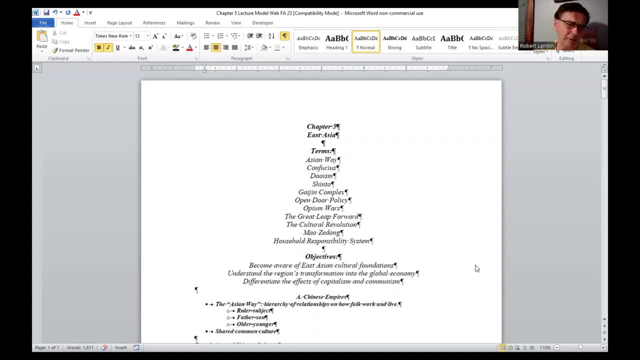 but many did under the cultural revolution. uh, maybe it was probably worse. uh, great leap forward. just stupidity of the system. the cultural revolution was, um, a calculated attempt to by the chinese government to eliminate opposition to the tune of millions. uh, that was under the uh leadership of mal zedong. mal zedong led the communist revolution in the late 40s. 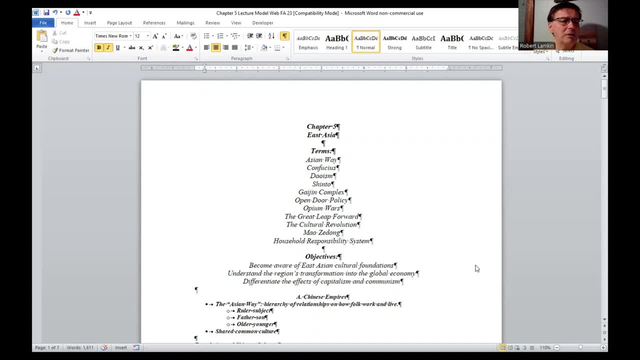 and the household responsibility system. household responsibility system- this was early on after mal died and the powers that be could see that they're going to have to make some types of um economic adjustments to get into um the wider world and not have the problems that they had with um part and parcel with the great leap forward and and uh. 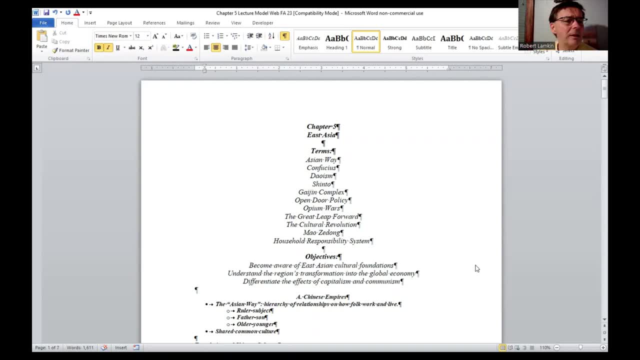 the bad economies that the chinese would have. and that was basically where the household responsibility system, where, when it came to agriculture, the government would let folks keep portions of what they grew and use it for. you know, evil profits, right. evil profits that the the uh communists um so decried and and hated, right. 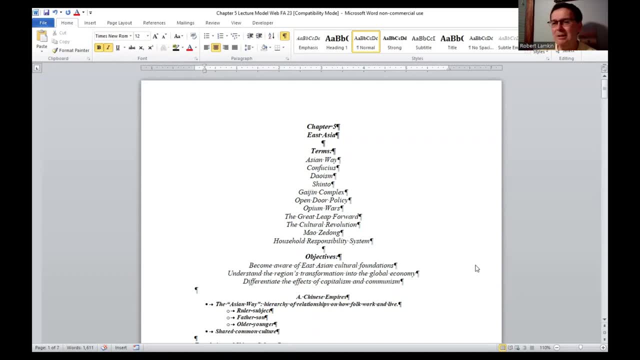 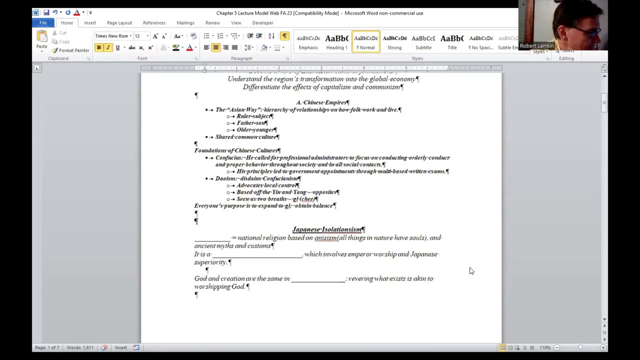 un�� in china, but they had, you know, in order to get the economy- Gesellschaft that generate ignorant money, uh, in a direction where it could be unself-sustaining, self-sustaining. so let's get into this. got some notes right off the bat. 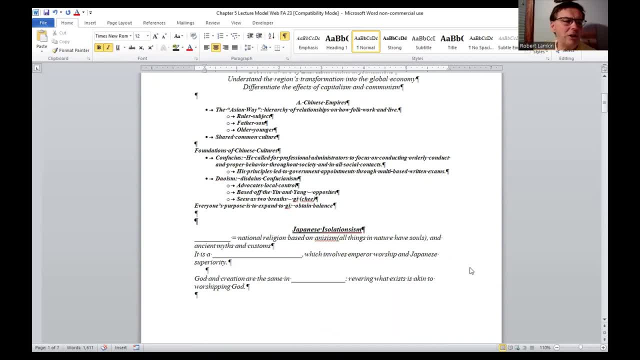 chinese empire. right chinese empire is the asian way, a hierarchy of relationships on how folks work and live. Ruler, subject: boss, employer, father, son, older and the younger. And this was a shared- it still is shared- common culture among the region. 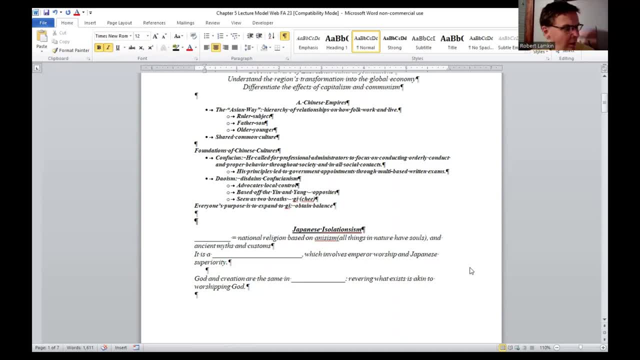 Then you have your foundations of Chinese cultures. You've got Confucius right. Confucius called for professional administrators to focus on conducting orderly conduct and proper behavior throughout society and in all social contexts. His principles led to government appointments through multi-based written exams. 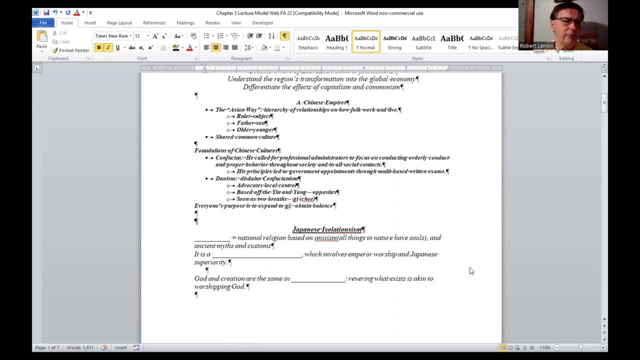 Taoism. Taoism disdained Confucianism. It advocated local control based off the yin and the, yang right Yin and yang opposites. the opposites seen as two breaths. the qi spelled G-I. 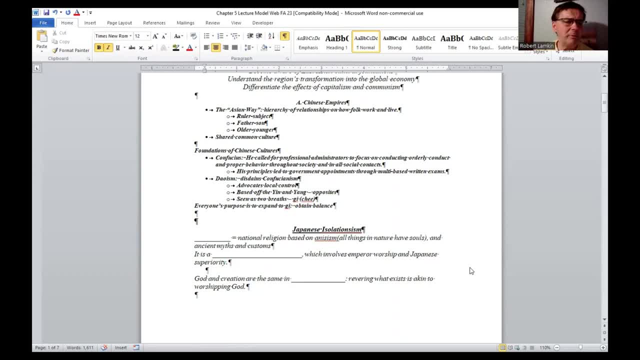 So everyone's purpose is to expand the qi, obtain balance, And you can see it even in the architecture. in China You have what they call male architecture, right, That is, you know, the part of the yin and the yang, the two genders, the male architecture and the female architecture. 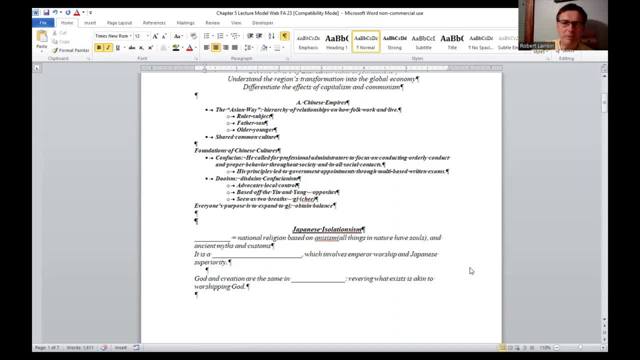 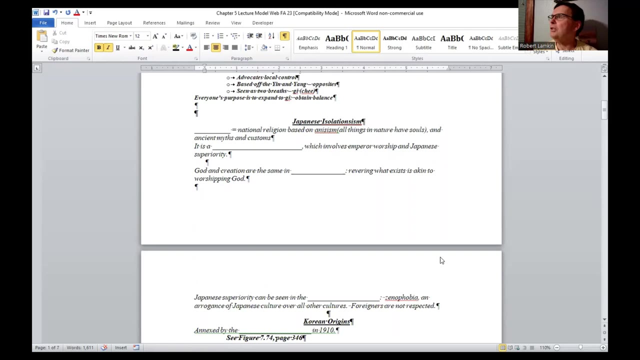 Trying to find that balance. The male architecture may be more pointed and the female architecture more rounded. soft colors And Shinto, Japanese isolationism. Now I'm going to be saying some things in here that are going to make me sound anti-Japanese. 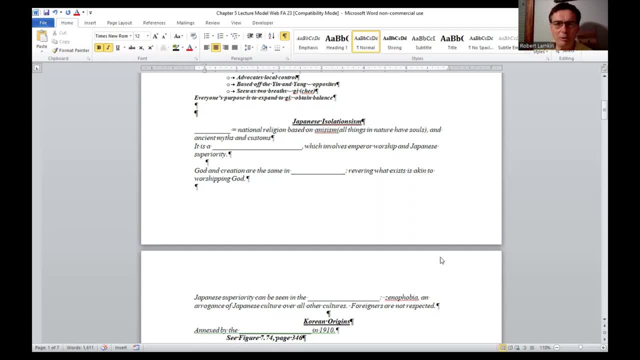 It's not that. I'm just telling you the facts about culture, right Culture and history, And you can do what you want with that. But Shinto is the national religion And it's based on animism. Based on animism. 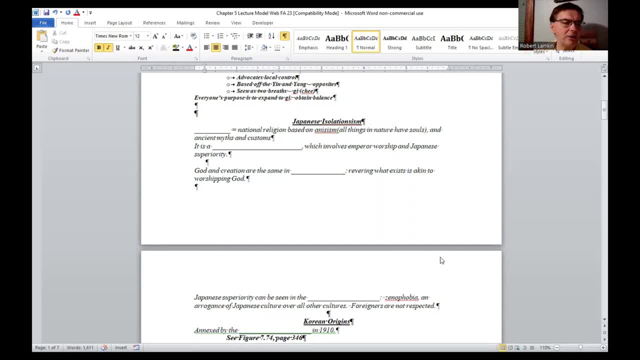 All things in nature have souls And ancient myths and customs. It's a pantheistic religion Which involves emperor worship and Japanese superiority. You can see figure 719, I believe it is. It's on page 293.. I'm having a hard time reading my writing between 9 and 8.. 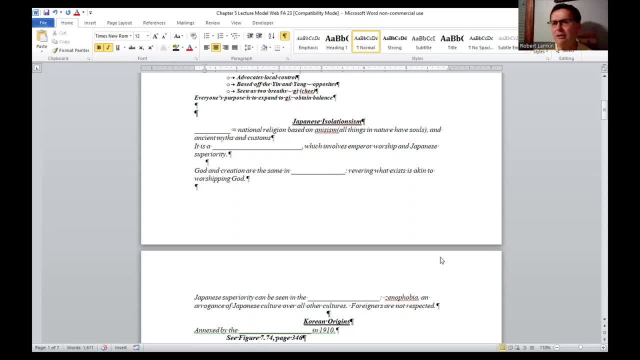 But if you turn to page 293.. You'll see if it's figure 718.. That's what I meant. 719.. That's what I meant. Okay, So yeah, It involves emperor worship and Japanese superiority. I'll just say something real quickly about that too. 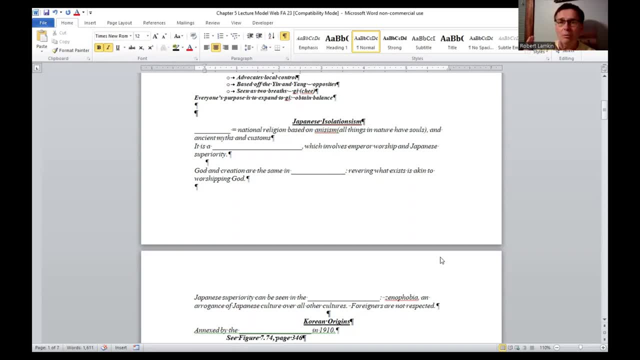 Kind of interesting. So emperor worship and Japanese superiority. So God is looked at In Japan as Japanese And the Japanese superiority bit. The Japanese went through a little nervous breakdown after World War II Because you know they didn't win right. 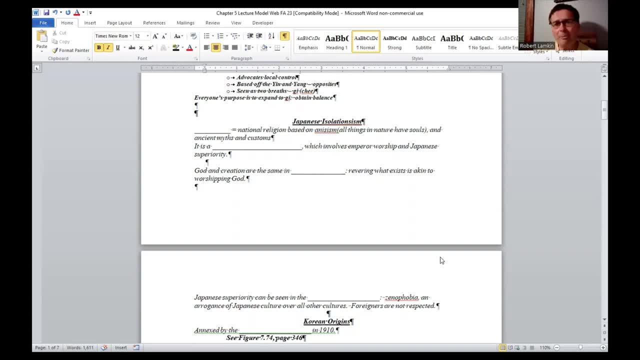 They lost, And they lost to. what I'm coming up here to Onto is a white foreigner, Okay. So I was like, hey, what happened? How could we have lost? We're superior, We're superior, You know. 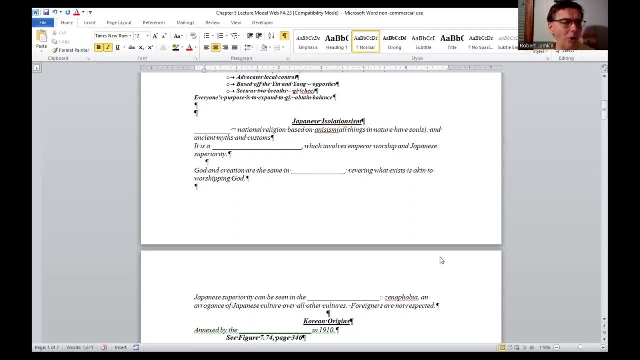 And to this white gaijin. So enter that concept here. Yeah, God and creation are the same in nature, And revering what exists is akin to worshiping God. So Japanese superiority. Japanese superiority can be seen in the gaijin complex. 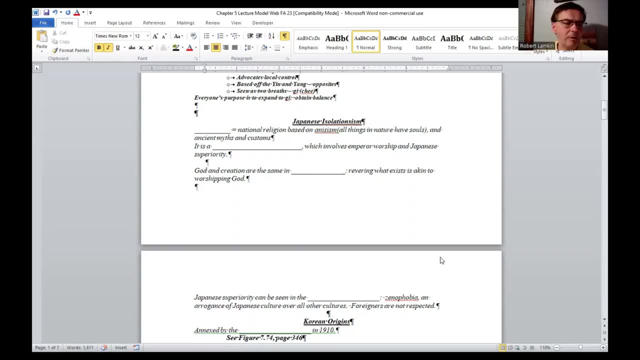 And that's one of your, And that's one of your heads up terms. It's xenophobia, right, And arrogance of Japanese culture over all other cultures. Foreigners, especially white foreigners, are not respected. However, because of the Japanese mindset of superiority, they have invaded and roughed. 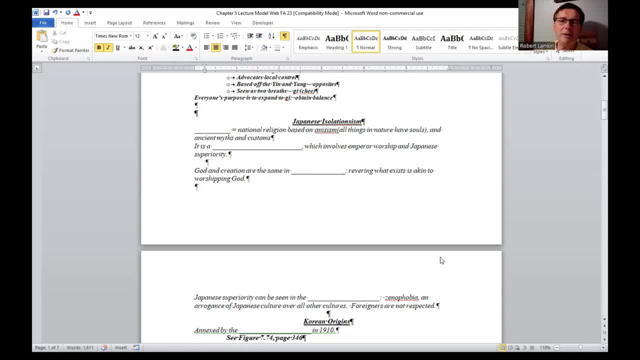 over neighbors for quite a while right. The Japanese are hated by the Chinese and the Koreans, and you know others in that region And in the next region that we're going to see as well. Let's take a look at Japanese isolationism a little more deeply here. 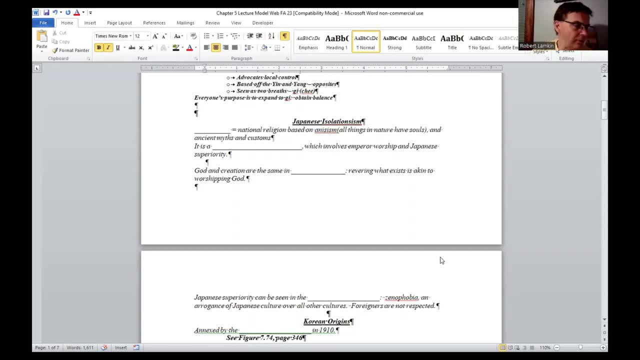 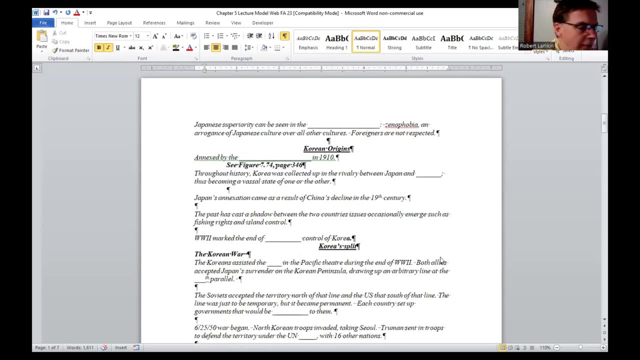 Japanese Japan's population. Yeah, Japan's population is about 98.5% Japanese, and it's probably the most homogenous society in the world, And it's widely believed that this has led the country to kind of a sense of purpose. 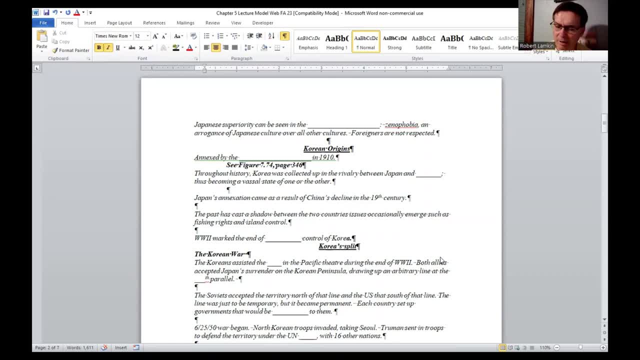 And there's so many other cool things about that I'd like to talk to you about, But I'm just not going to have the time to do it. So let's take a look at Korea. Korea was annexed by the Japanese in 1910.. 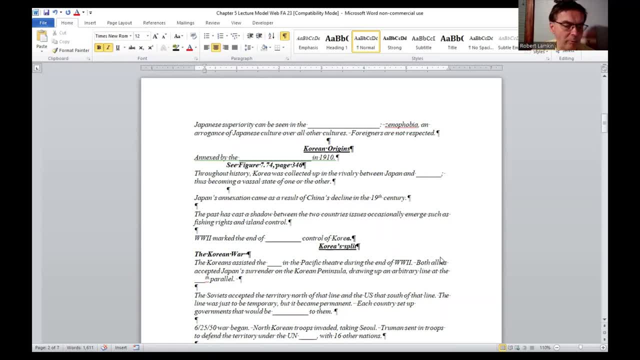 And you can see figure 774 on page 346, page 346, and kind of curious about what I was looking at there, What I want you to see, And yeah, just a map, right, an overall map of the region. So, yeah, you want to keep a keep a mark bookmark in there and turn to that as we need to. 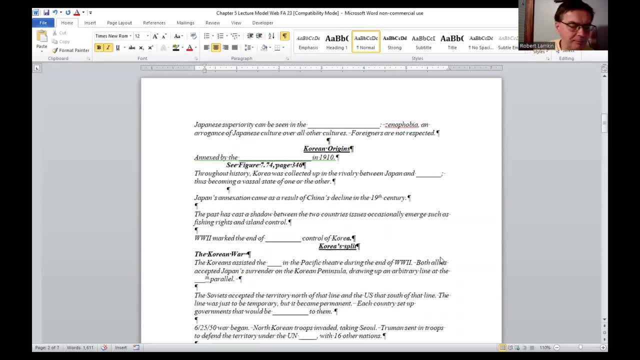 But yeah, right, This is geography, We need the maps. So, throughout history, Korea was, as I say, collected up, right, collected up. So what's the history of Japan and China in the past? Well, Japan, Japan, was a state of one or the other. Japan and China are two independent states. It's not like you know. it's not that they were the only two countries that were in conflict when Japan came along right. There was a period in time you know that Japan really did not have a very highanding 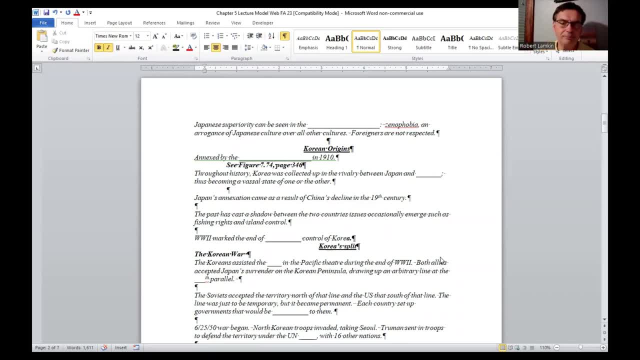 position in the country that really was pendant among the Japanese, And it hasn't been that long since. so, But if you think about it, the relationship between Japan and China- what happened was that Japan began to form one of the most important allies in the country in the last 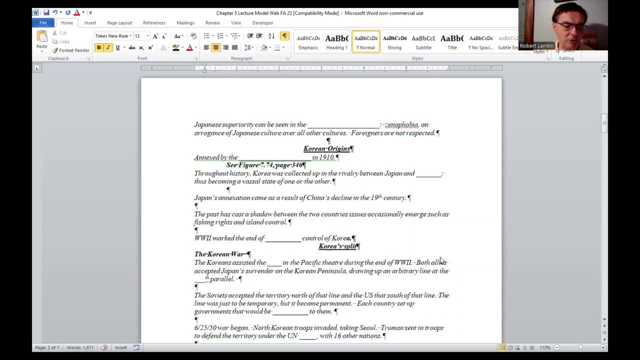 decade. That's the period when the entire democratic system of Japan started to become the part of a economic process, And Japan then came to the United States and the other two countries. in the last decade. China's decline in the 19th century And the past has cast a shadow between the two countries. 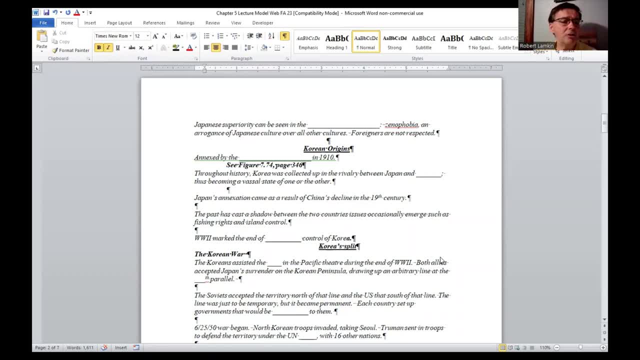 Issues occasionally emerge, such as fighting rights and island control. World War II: as I said, World War II marks the end of Japan's control of Korea. Korea split: let's take a look at Korea split 1950, the Korean War right. 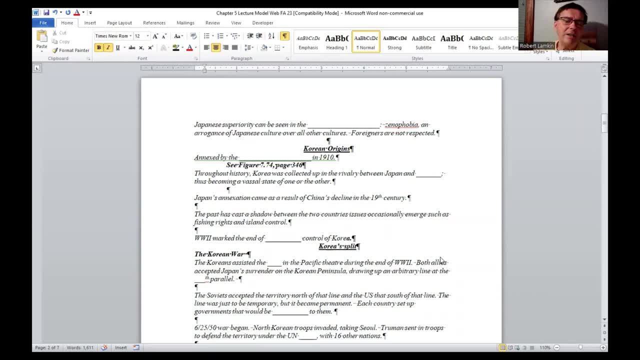 Korean War. they assisted the United States in the Pacific Theater. during the end of World War II, Both allies accepted Japan's surrender on the Korean Peninsula, drawing up an arbitrary in the line at the 38th parallel, Again on page 346.. 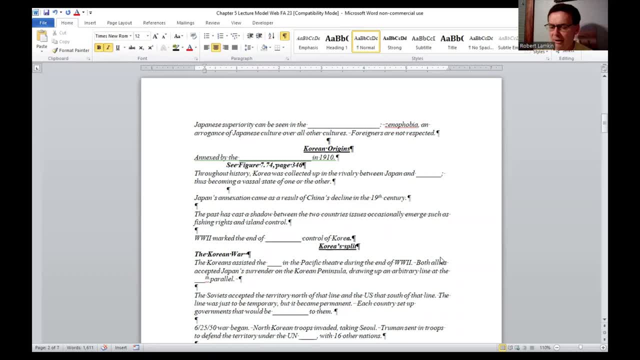 It would probably behoove you to take a look at, find out where the Koreas are- North and South Korea- and look at the divide, the division there between North and South Korea. Just above Seoul, you see the shaded color of North Korea, and that would be the 38th parallel. So the Soviets- and this is during the Cold War- the Soviets accepted the territory North of that line and the United States the area south of that line. So the line was just to be temporary, but it's become permanent right. Each country set up governments that would be friendly to them, right. So, North Korea, you have a communist government. June 25th 1950, the war began. North Korean troops invaded, taking Korea. They took Seoul. Truman sent in troops to defend the territory under the UN flag, with 16 other nations. And just kind of going back at World War II, right, The Soviets were allies of ours, and so there was an agreement made once the shooting stopped, that, you know, Soviets were, you know, very interested in that territory too, that peninsula. 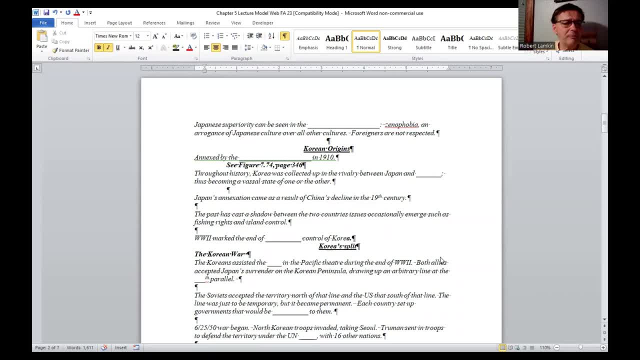 and we divided it up right Along the 38th parallel. So yeah, Truman sent in troops to defend the territory under the UN flag with 16 other nations By September of 1950, General Douglas MacArthur right, he jammed the advance all the way back. 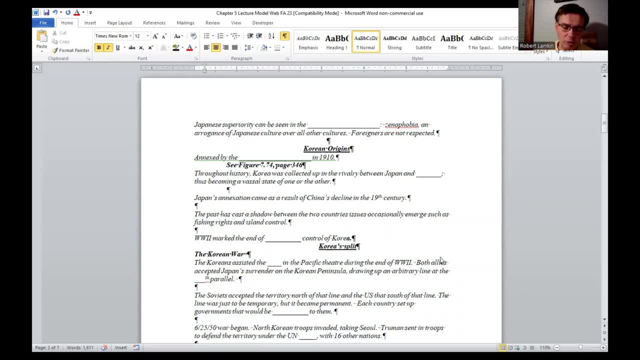 to the Chinese border at the Yalu River and you could see just north of northwest of North Korea, the border of China, and you could see the Yalu River there And Lost- kind of lost- my place there, Oh yeah. 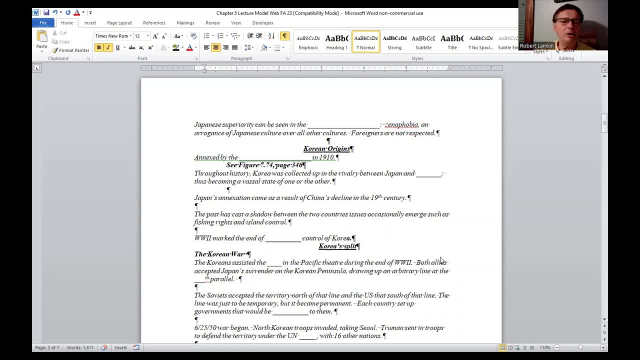 Apologize for that. Yeah, so all the way up to the Yalu River, and MacArthur at that time. he stresses using nukes, right, He stresses nuking, every nuking the area Truman resists, right. 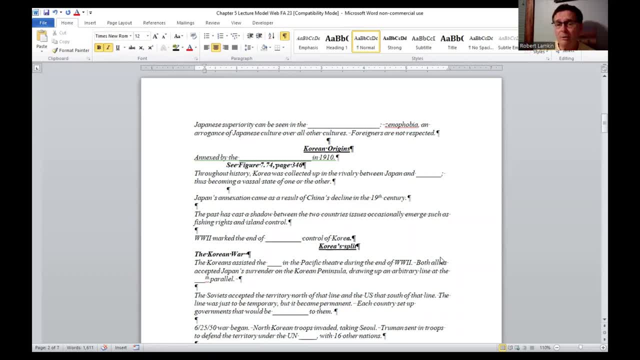 Truman's the commander of the chief commander-in-chief, And so MacArthur's got a little problem here because MacArthur doesn't agree with him and MacArthur went ahead with bombs and Truman sacking right. A lot of Americans at the time were disappointed in MacArthur. 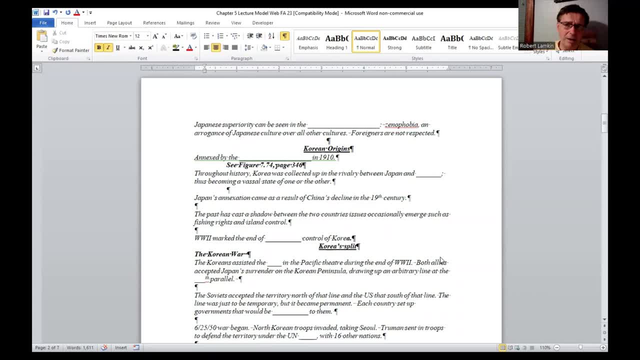 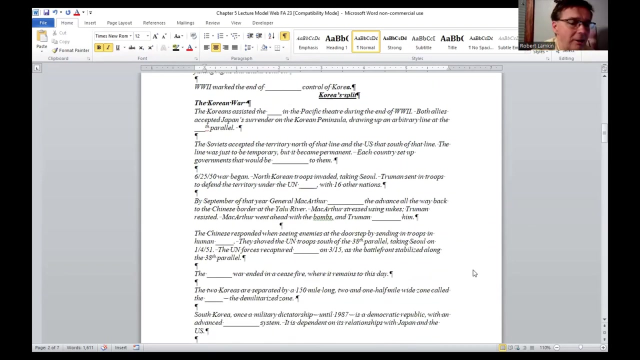 but I think over time recollection has been kinder to MacArthur and his position. the chinese responded: right. the chinese responded when seeing enemies at the doorstep by sending in troops in in human waves, to be quite um graphic about it. um, so they shoved the un troops south. 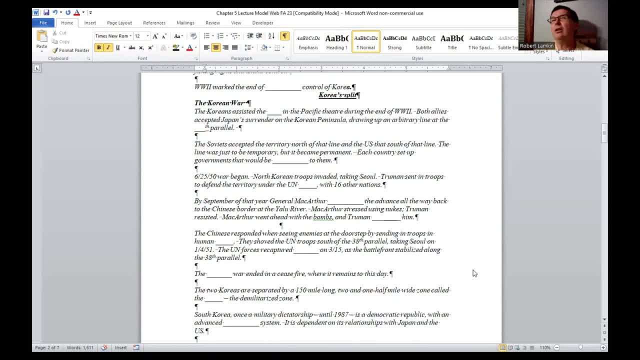 of the 38th parallel, taking seoul on january 4th 1951. the un forces recaptured seoul two months later, as the battlefront stabilized along the 38th parallel. so this proxy war ends in a ceasefire, where it remains to this day. right, the war is ongoing. right, we, we need to finish it. 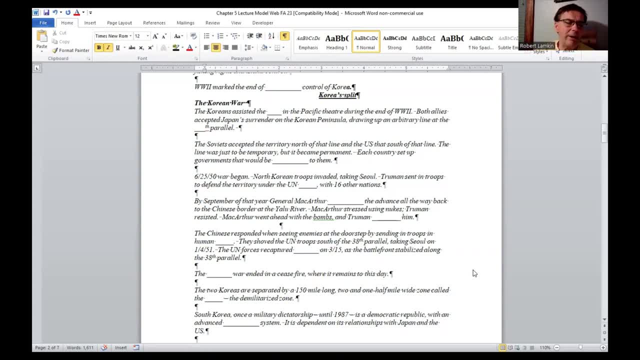 so the two koreas are separated by a 150 mile long, two and one half mile zone called the dmz. so again, you look at the boundary, the dmz, and picture this. you know a 150 mile, uh wide, uh long barrier, two and a half mile wide zone called 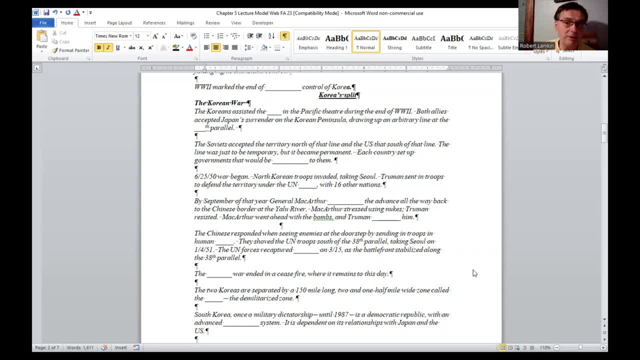 the dmz, so it's called the demilitarized, demilitarized zone. south korea was uh once a military dictatorship until 1987 and it is um now now a democratic republic. now, democratic republic uh, with, uh, i might add, an advanced capitalist system. so, but it's dependent. 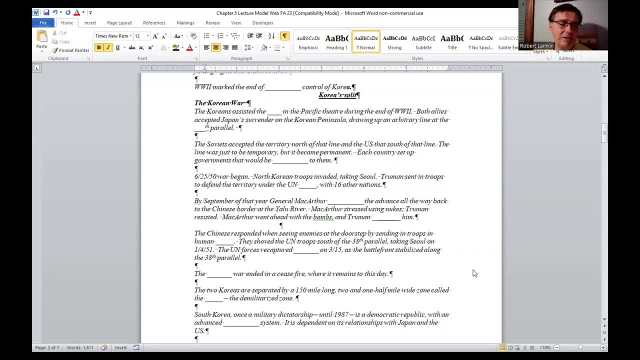 on its relationship with japan and the united states. north korea, as we know, is a police state, uh, promoting what it calls a juche, right juche. so what's up with the uh juche? well, basically, um, north korea wants um to be self-reliant, right, they want to be self-reliant. 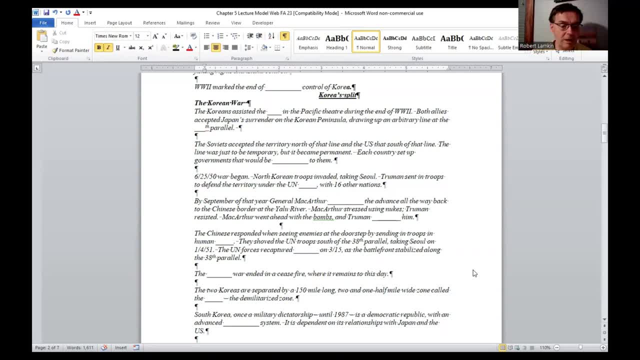 and um you know, not reliant on um certainly any of the um you know neighboring, um neighboring areas. so you know, juche, um you know independence, right, they want independence um be self-sustaining, um have a national self-defense and, yeah, again, complete limitation from the. 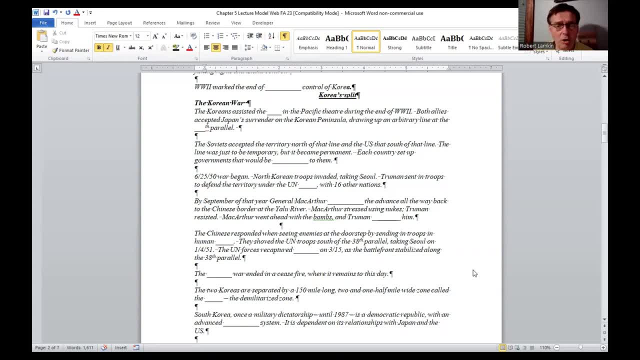 outside world. it's in fact north korea, as is called uh the world's hermit right. so responses from this area, responses uh to the um outside, outside world and um. beginning in um the 1500s, the portuguese led european expeditions to the region. china resists any kind of colonization. 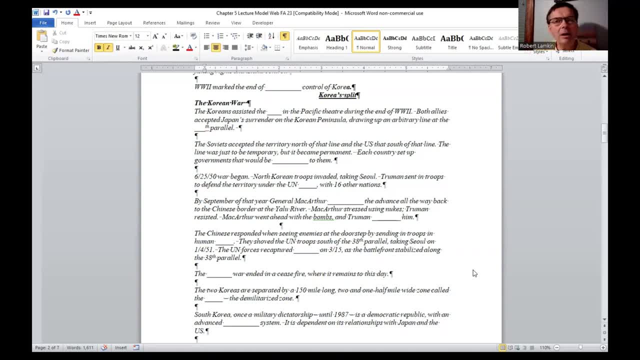 demand for chinese tea comes through the british east india company. uh, the brits traded opium at the southern port of ghana jiao, and you could see a poster on page 297, a poster, uh, that was um, published in 1900, figure 723, and in this political cartoon, 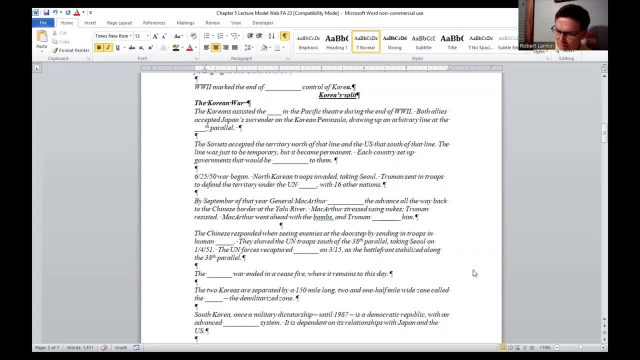 colonial powers are seen dividing up china under the enraged but helpless qin dynasty. from left to right, you got queen victoria of great britain, kaiser wilhelm of germany, the czar nicholas in russia, marianne as the emblem of france and a samurai soldier representing 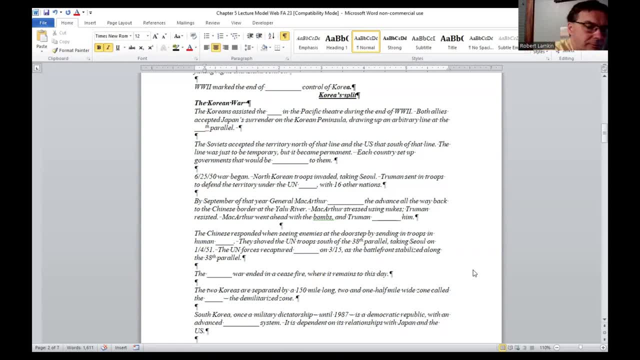 japan qin government forbade the opium trade and it starts the opium war of 1841- 1842. um what happened there? was confiscated uh british opium uh ends up into a murder of a chinese port authority by british and american soldiers. um the war was confined to a particular area, uh, to canton and east- some of the east uh. cities uh as far north as tangin. uh british the britain, uh the brits do threaten nanjing and uh the qin dynasty eventually sues for peace. and this is at the juncture where um, shortly thereafter that the british uh gained hong kong. uh hong kong about, i guess, about 40, 50 years later. 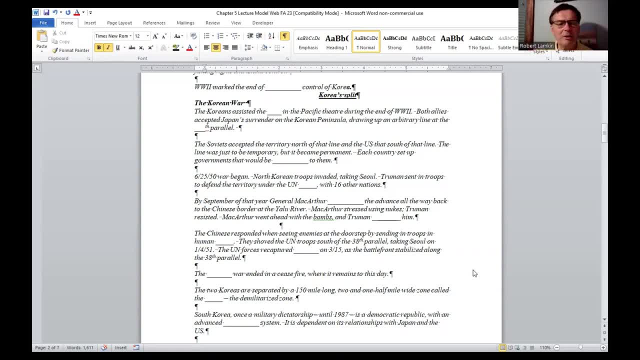 japanese aggression. right again, i don't want to sound harsh, don't want to sound anti-japanese. uh, during the 1800s, uh, the japanese build a military to counter this newfound western aggression. they begin to modernize. they begin to modernize for economic stability, which leads to trade, uh, 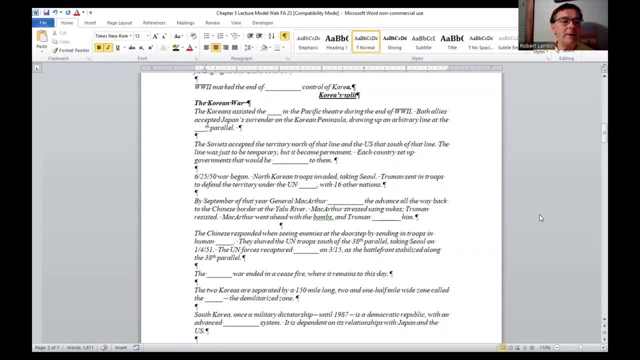 mediocre goods, right. they democratized in the 1900s and they set up an internal pact between the japanese military and the japanese elite, who at the time were the zabutsu family, and uh, that family owned all of the jerusalem capital. uh, japanese, uh big industry, right. so this, this combats against japanese goods. 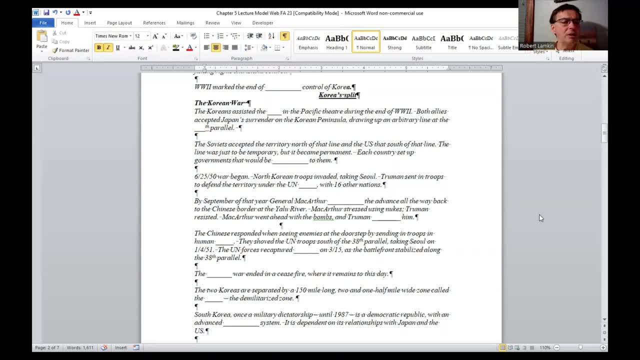 and this leads to, uh, world war ii because the japanese invade china, and uh, they made the manchuria area to be specific, a lot of copper and other resources in that region and uh, you know, gets the west nervous and, um, you know, and they do this because they see themselves as the 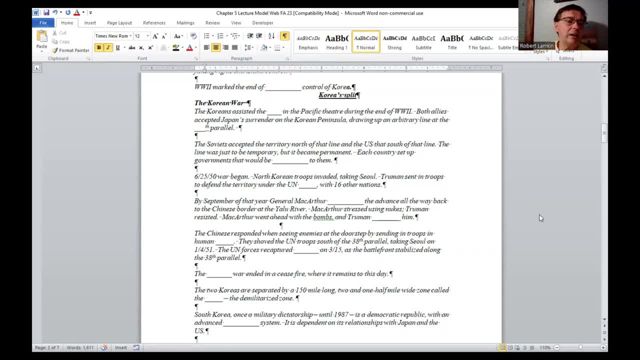 superior race. world war ii changes a lot here, changes a lot of um japanese confidence. i guess you could say: turn to page 277. i want to just look at the physical environment here momentarily. and um 277 you have east asia's physical environment and it's very uh, very uh diverse. you have human climate, rain. 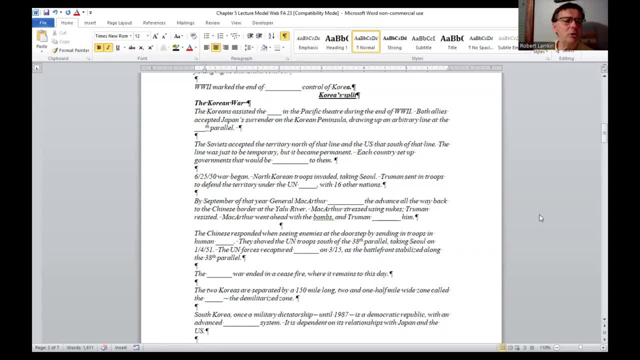 climates ranging from coal mid-latitude in the north the subtropical and tropical in the south. you got mongolia and western china are dominated by arid and semi-arid climates. the region has a substantial and diverse natural resource base. um much of the region is mountainous, with much of the larger lowlands concentrated in eastern china. 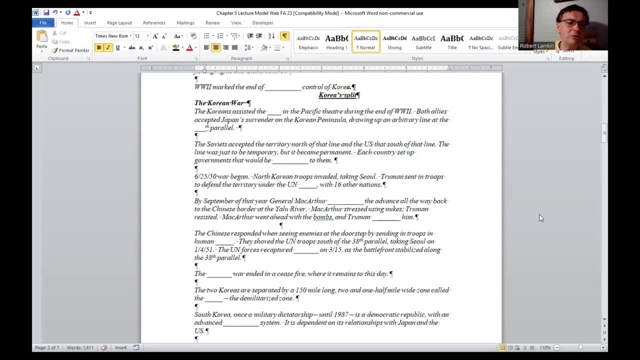 you got high mountains and plateaus that dominate western china and serve as a headwaters for many, uh many, many of the um, many of the rivers, okay, active plate boundaries in the region, so it's fairly seismic activity. some of the world's worst earthquakes have located, been located in that particular particular area. 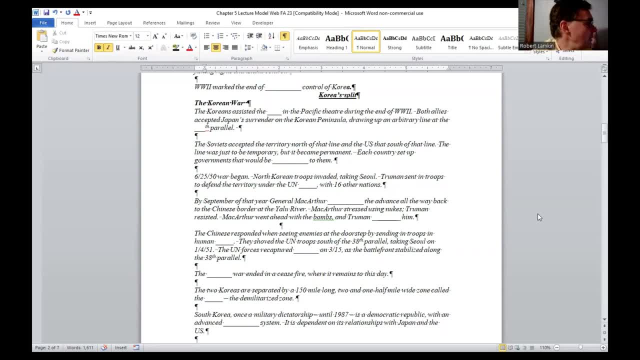 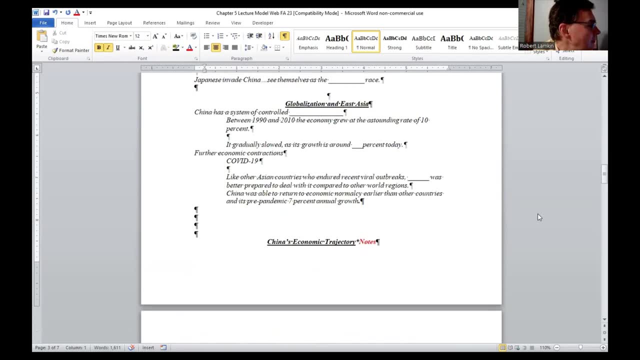 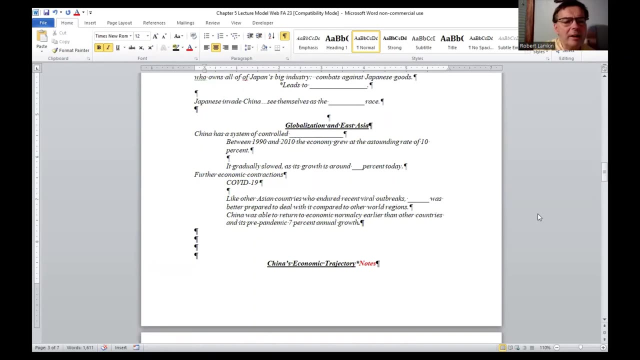 i want to take a look now at china's entry into the global economy: globalization in east asia. china has a system of controlled capitalism and a lot of times you'll hear the word we throw these words around irresponsibly. you'll hear the word fascism. right, he's a fascist. fascism is. 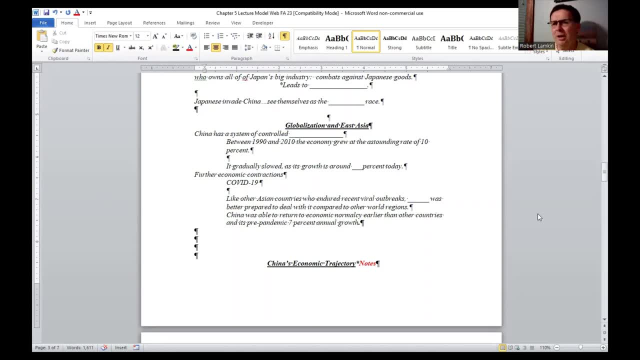 basically um hitler and the nazis did. it was, uh, controlled capitalism. controlled capitalism, uh, and i i would strongly argue that's what china is today. very, they're communists, but they have a controlled free market system. so china has a system of this, and between 1990 and 2010, the economy grew at the astounding rate. 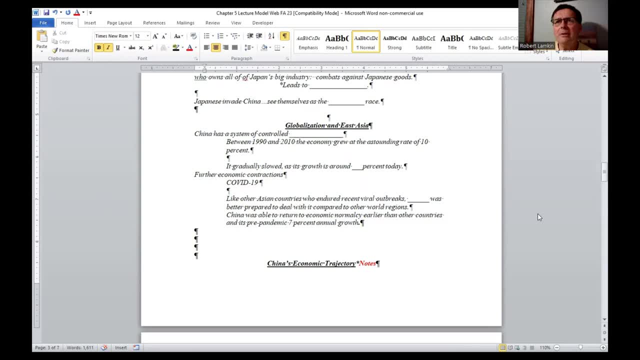 of 10 percent um. it gradually slowed as its growth now is around seven percent. but let me just say something about that seven percent growth. most people around the globe would die for that right. that's. that's good growth. um further economic constant contractions were due to covid 19. like other asian countries who uh endured these uh viral outbreaks, china was um better prepared to deal with it compared to other regions, quite frankly, and so, therefore, china was able to um return to economic normalcy earlier than other countries, and it's pre-pandemic seven percent annual growth. 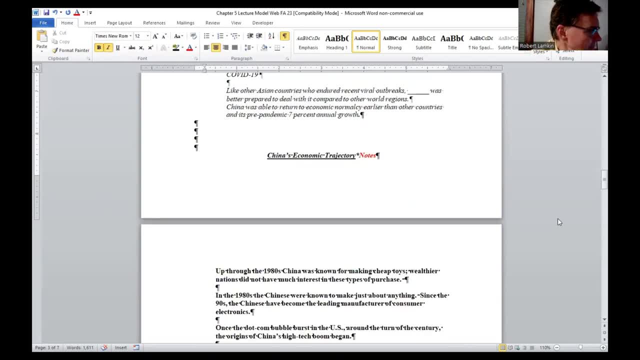 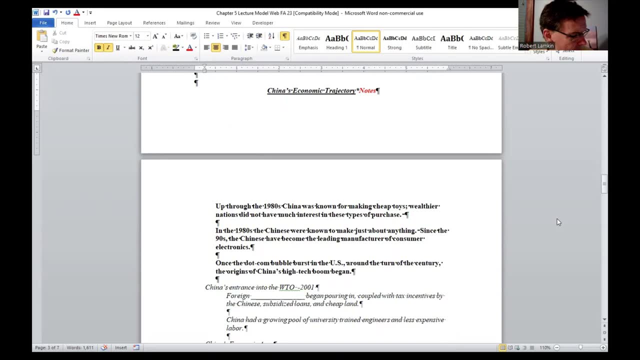 china's economic trajectory. up through the 1980s. china was known for making cheap toys. uh, wealthier nations did not have much interest in these types of purchases, so in the 1980s the chinese were known to make just about anything. um consumer electronics, um, they became the leading, leading manufacturer of that. 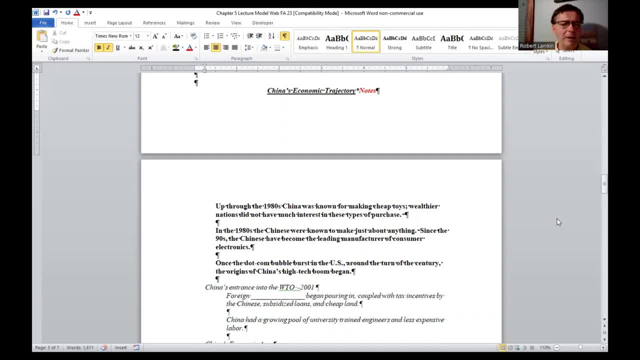 um, probably since the 90s. uh, page 301 in your uh textbook. i have you guys turning to that and yes, there is a figure 726- apple products, apple product factory there. right, a young lady there, um, i don't suppose that she's smiling for the camera, but she's not. but anyway, you can look at that um. 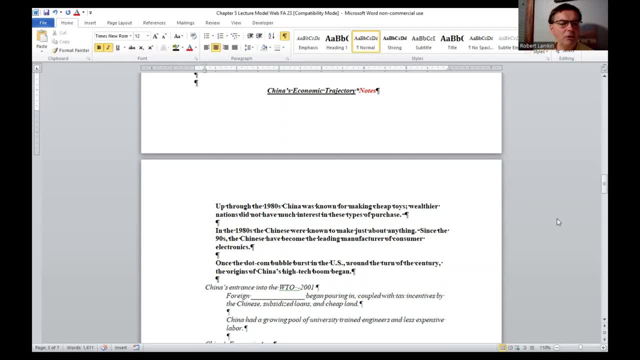 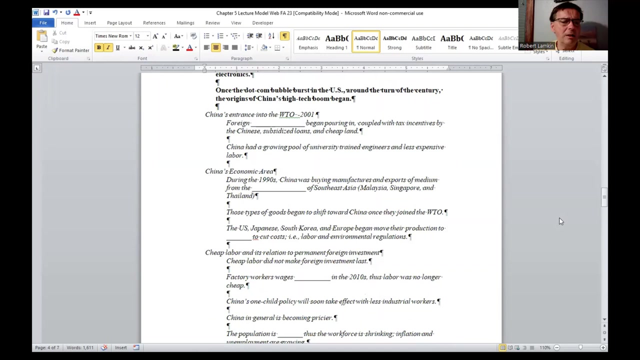 check that out. so what's? the dot com bubble verse in the united states around the turn of the century. that is where the origins of china's high tech boom really begins. china's interest in the world trade organization 2001: a foreign investment right. because of what? 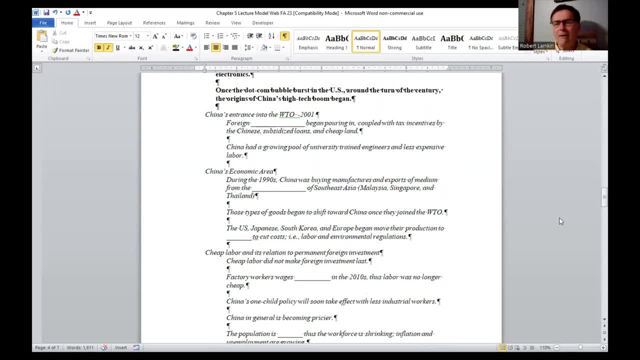 i'm talking about begins pouring in, coupled with tax incentives by the chinese, subsidized loans and cheap land. china had a growing pool of- also of university trained engineers and, you know, less expensive labor. china's economic area. well, during the 90s, china, china was buying up manufacturing manufacturers. 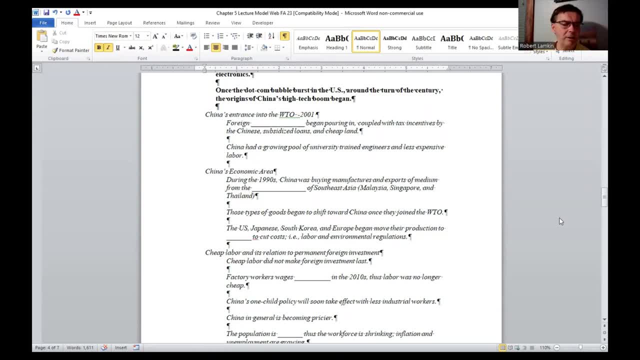 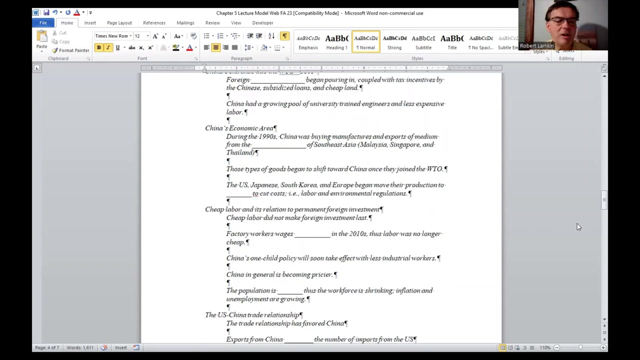 and exports of medium from the asian tigers of southeast asia, malaysia, singapore and thailand. we'll get to them next and they really boomed during this time. so those types of goods begin to shift toward china once the chinese join the um wto, so the united states 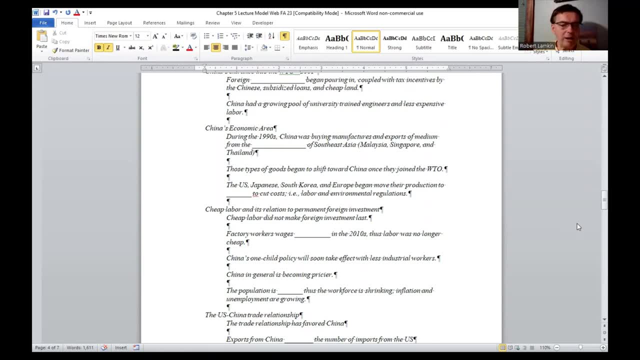 the japanese and south south korea and europe began moving their production to china to cut costs. um, you know, ie labor and environmental regulations, cheap labor and its relation to permanent foreign investment: um, cheap labor doesn't seem to have made foreign investment last. uh factory workers. their wages doubled in the 2010s, so you know. 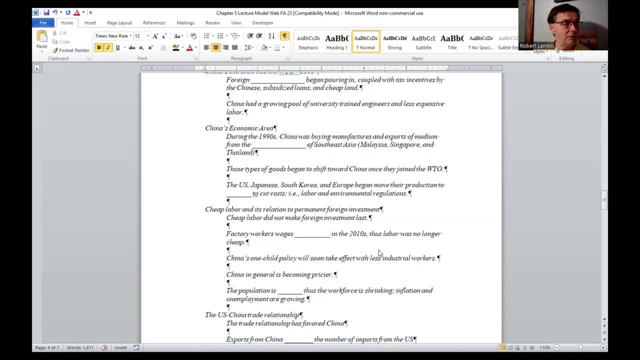 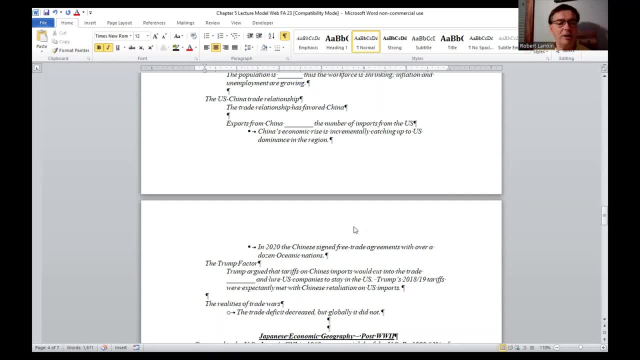 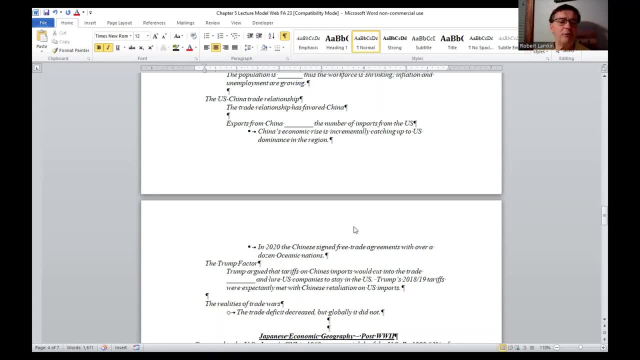 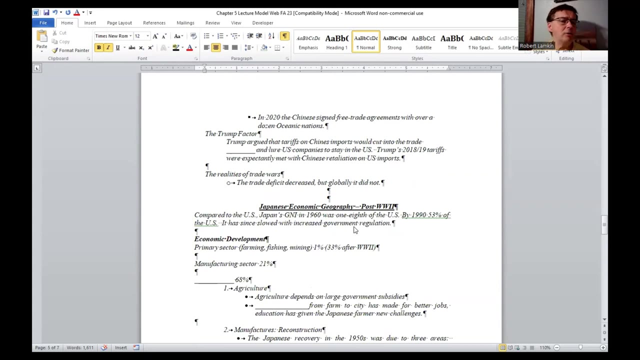 the chinese signed a free trade agreement. well, several free trade agreements, umm former trip now. uh institutional structures and restore banking. that you have a traditional father, uh, literal. but just having one child could mean a lot of dough. Högland and款 and聯овых ficengard 웃음. 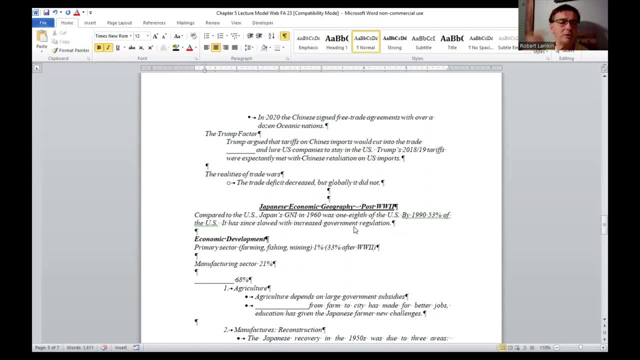 would cut into the trade deficit and lure us companies to stay in the united states. his 2018-19 tariffs were expectantly. i knew this was going to happen. met with chinese retaliation on our imports, so what were the realities of these? then becomes a trade war, and the realities was: 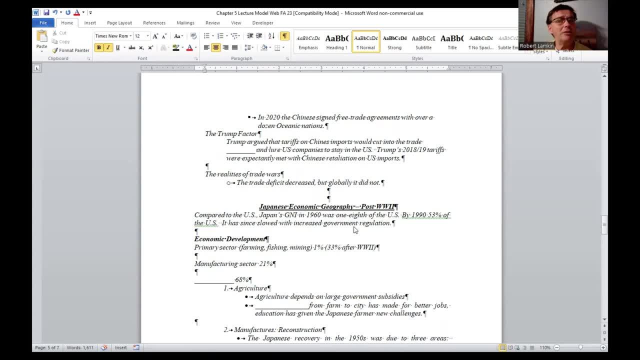 that the trade deficit between the us and china did decrease and china- and, uh, mr trump did have that right about the. you know we were kind of taking the cleaners on certain things, but globally it doesn't. it doesn't really do anything right. the reality of the trade wars it. 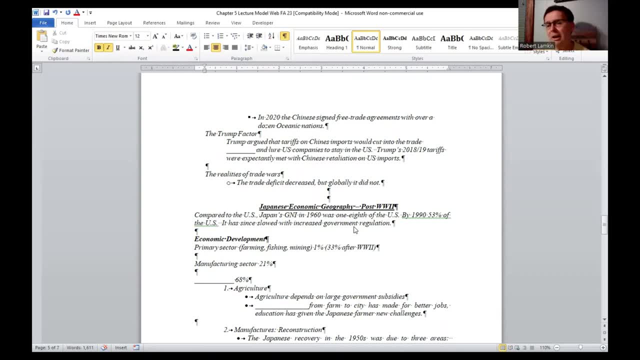 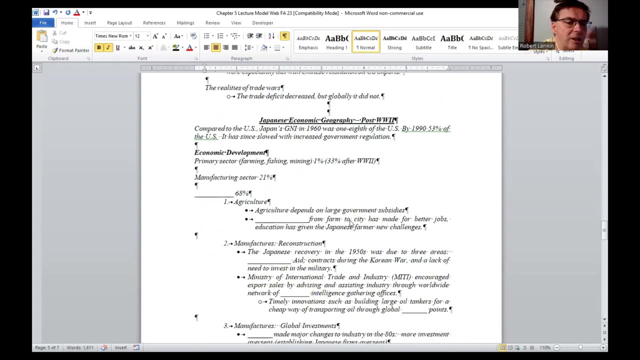 doesn't, doesn't help anything globally, and maybe that- and i don't think that was um, you know president, you know president, you know president, trump's um goal? uh, in the first place, japan's economic geography. all right, japanese development compared to the uh us, the um japanese, 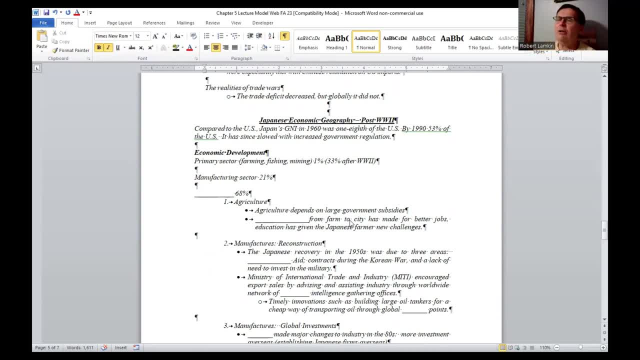 gni gross national income in 1980 or 1980 was just one-eighth of that of the united states. by 1990 it was uh. by 1990 it was 53 percent of the us and it has since slowed with uh, increased government regulation. 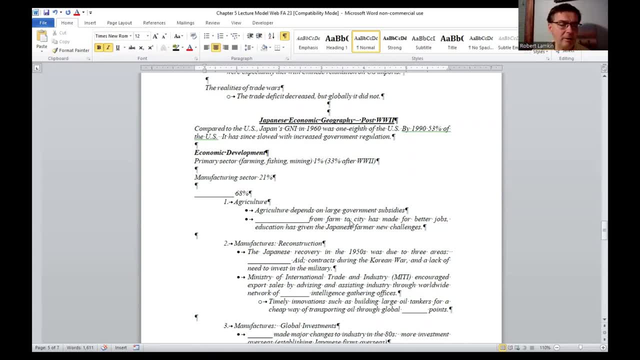 economic development. the primary sector where you're just you know, you know, fishing and mining and farming was uh is at one percent with the us and china and china's economic development is is at about ahimiseock's uh course in the recent happenings. world war one uh development sector was actually thirty-three percent after world war too uh, the manufacturing sector is also a dropped to twenty-one percent um the service sectors at about seventy percent of the japanese economy. agriculture still uh depends on a lot of large 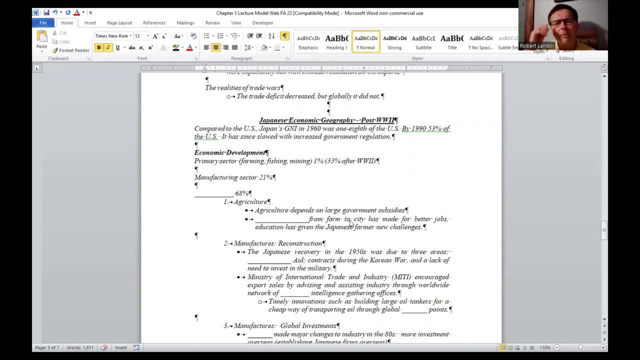 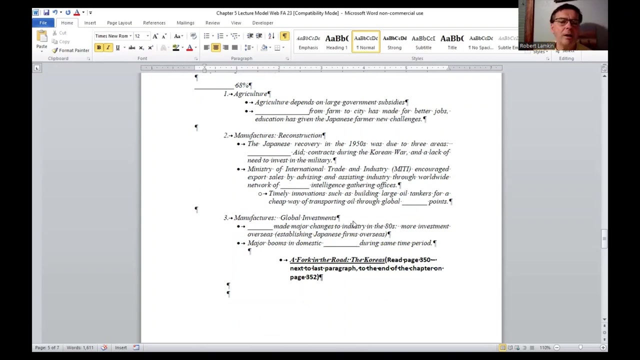 uh government subsidies, true, true perp. The farm, the city has also made for better jobs. Education has given the Japanese farmer new challenges, Manufacturing reconstruction. The Japanese recovery in the 1950s was due to three areas: American aid contracts during the Korean War. buses and our bases and airports, and a lack of need for the Japanese to have to invest in the military. They were being protected by the US. So these are the three areas that really allowed the Japanese economy to boom And, of course, the gaijin right. 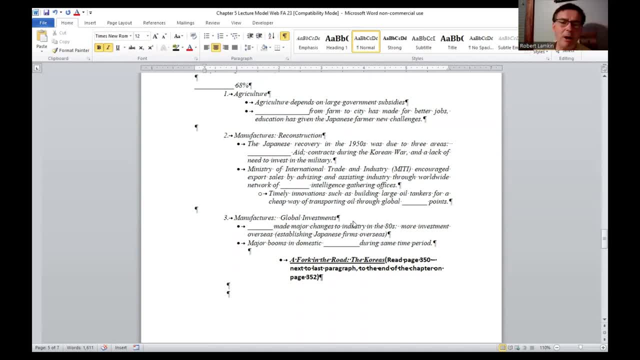 We are remaking Japan in our own image in the free market, democracy right, The military of international trade and industry, the MITI in Japan that encouraged export sales by advising and assisting industry through a worldwide network of market intelligence gathering offices. So with that you had these timely innovations, such as building lines, building large oil tankers for a cheap way of transporting oil through global choke points, like you know: the Panama Canal, the Strait of Hormuz, the Suez Canal. Manufacturers, global investments. Japan made major changes to industry in the 1980s: More investment overseas, establishing Japanese firms overseas. Japan made major changes to industry in the 1980s: More investment overseas, establishing Japanese firms overseas and major booms in domestic retailing. 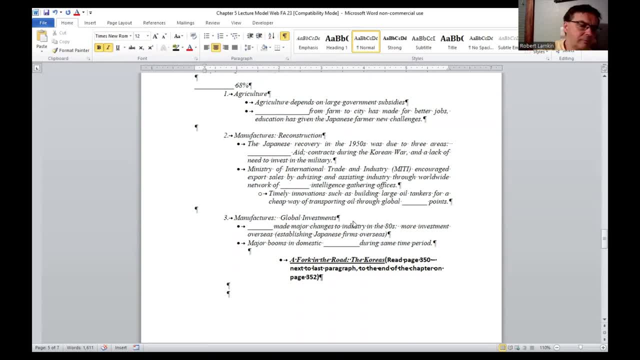 during the same time period. Take a look at your textbook again, your map there, page 346,, figure 774, and I want you to zero in on that island called Japan, Because I want to say something about the population and, uh, some of the advantages and disadvantages of that island, the size of it, um, the nation's. 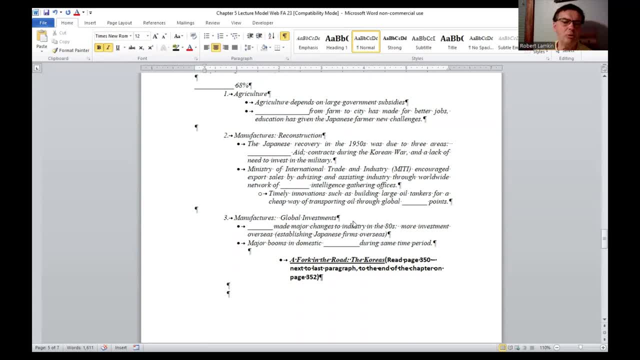 dramatic economic growth after world war ii. uh, their defeat was one of the 20th century's more incredible feats, otherwise known as the japanese miracle. so you had wise investing in industry and industrial plants. the political culture, the ldp, the liberal democrat democratic party, has been the sole ruling party since 1955. um, conservative, it's very conservative and it's. 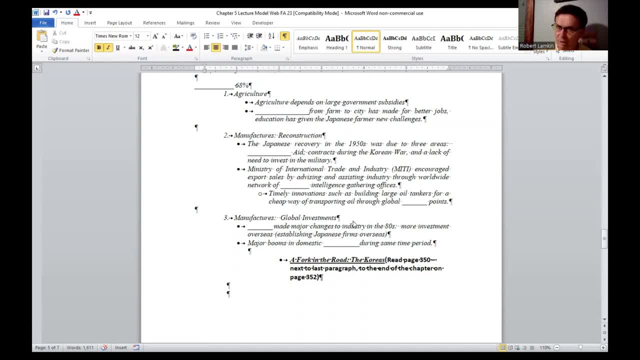 business friendly, uh. it cooperates with the business community in new products and new industries. the relationship between politicians and business, um what we would call crony capitalism- seen elsewhere in southeast asia, which we'll look at next, has been to blame for the erosion of japanese growth. 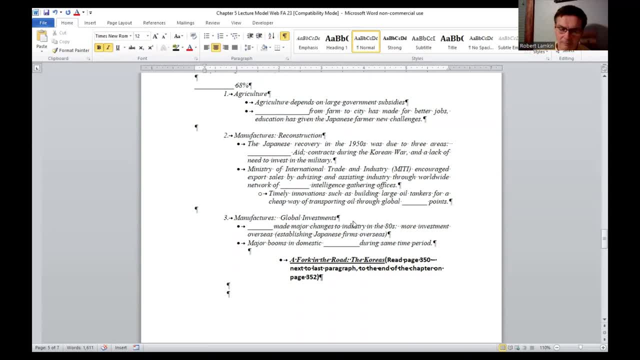 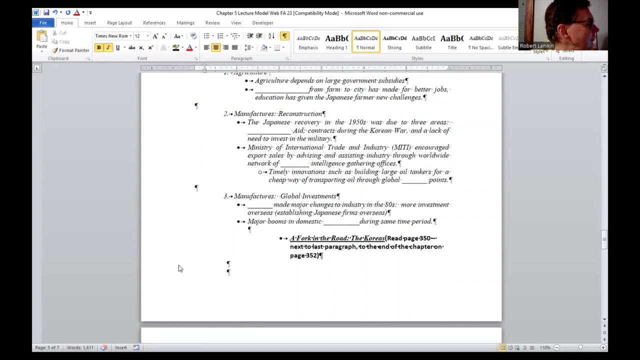 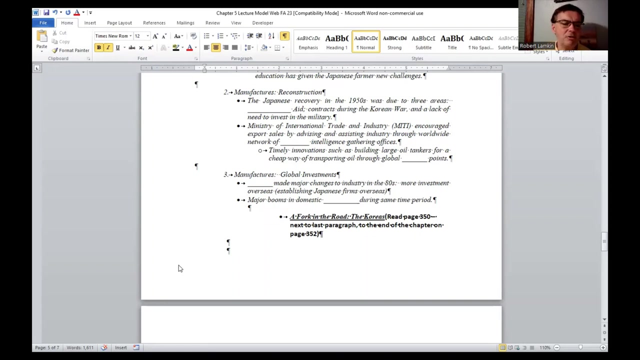 if there's anything i want to say on that- the rise and fall of the um, um japanese economy- again a lot of good stuff there, you just don't have time to do it. i would say this: um, despite the problems, japan's economy is the fourth largest. 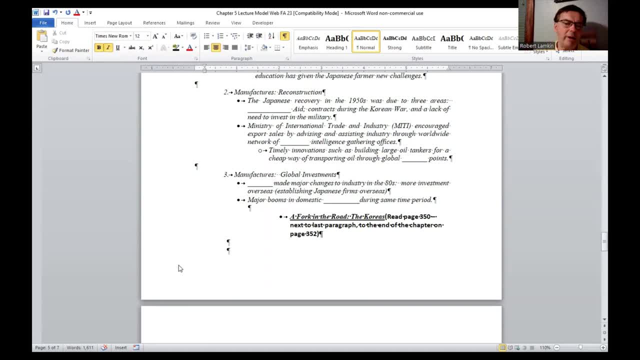 in the world. it's uh trade surplus and low rates of inflation, uh, and unemployment as a result. you got major companies there such as toyota, honda, nissan, and they have global business right. you got sony, panasonic, nintendo, that make, uh, you know, japan, the world's preeminent uh electronics industry. okay, so 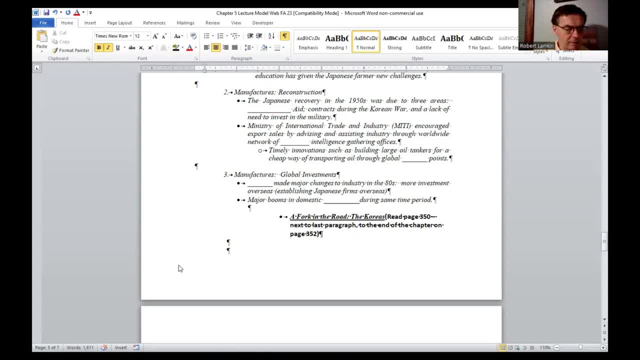 you got that uh with, uh with japan. so i want to go to next here. let's um, take a look at um. go back to china. go back to china, oh, um, korea. i want you to um, this is in your readings: a fork in the road to korea's. uh, we looked at you know what happened? we looked. 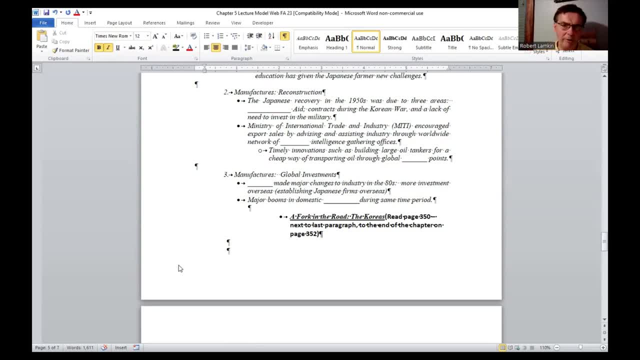 at the korea war, korean war and the split between the north and the south. because of time, i want you to read pages 350 to the next, to the last paragraph, to the end of the chapter, on page 352 on that, because that stuff's gonna. information will show up on the quiz and and so forth. so you're going to need to read that. china collectivization and the communes in 1949 trying to begin to model its changes. uh, on the soviet model. after the chinese took the took over a large social investment in the industry, not too much in agriculture, right. 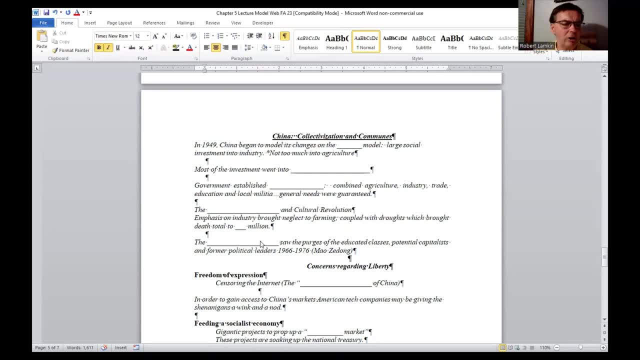 they're copying those five-year plans of joseph stalin looking to industrialize. most of the investment went into manufacturing. obviously, government added communes: right. combined agriculture, industry, trade and education. local militia, general needs were guaranteed right. the communist system was underway under these communes. the great leap forward. and here's some of the results. 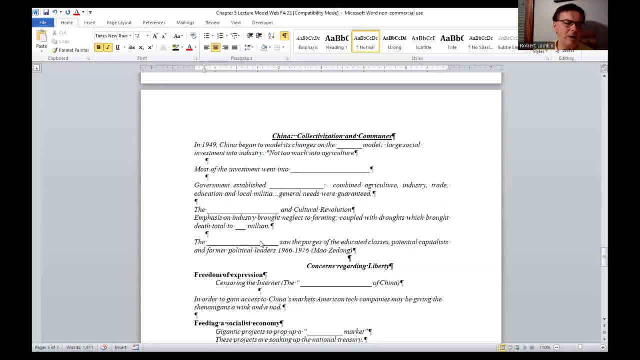 of just the mismanagement of the communist system. the great leap forward and cultural revolution. you had a emphasis on industry that brought a neglect to farming coupled with droughts, brings about a death total of 30 million people. i mean, how sad does it get right? cultural revolution saw the purges of the education, educated classes of Great Leap Forward was 1959 to 1961, you know, 10 years after the Communists took control of Cultural Revolution. 1966 to 76. right up on the eve of Mao Zedong's death in 1976, the Cultural Revolution saw the purges of the educated classes, uh, potential capitalists. 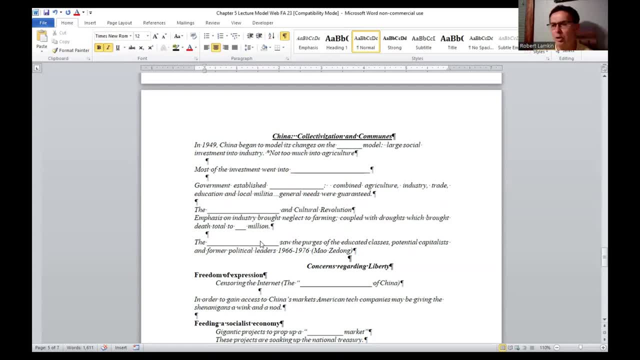 and former political leaders, to the tune of just millions of people, right, uh, dying. so the question: where does China go right? where to now? uh, China? a lot of people wonder because of the um, you know, some of these heavy-handed uh abuses and um, you know, how is that going to um, how's that going to work, right? well, where to China? I've. 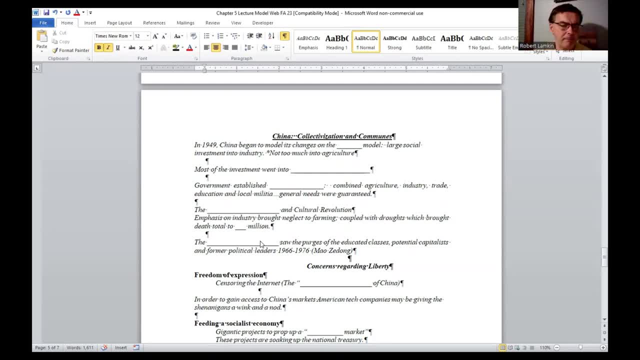 dubbed this here: concerns regarding Liberty right: concerns regarding Liberty freedom of expression right. freedom of expression expression. the Chinese government censors the internet right, otherwise known as the uh great uh, the Great Firewall of um of China. so, in order to gain access to China's markets, American tech companies may be. 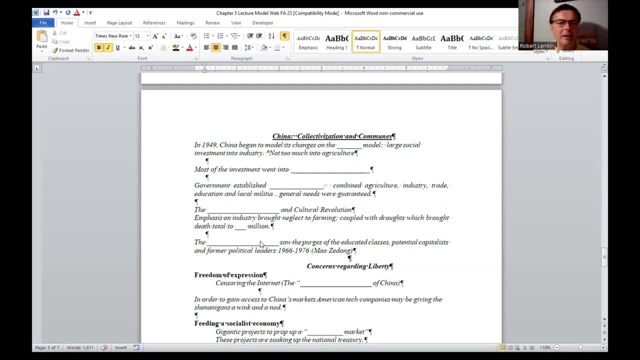 giving the? uh, all this tomfoolery and these shenanigans? um, they might be ignoring it. right, I think they might be ignoring it. uh, the the NBA? um, they are making a lot of money in China. they have people like LeBron James has failed to use. 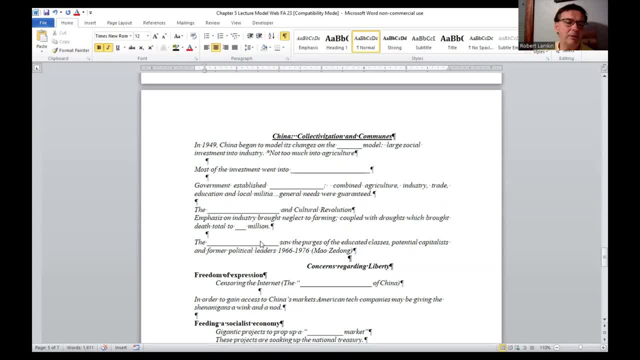 a social platform, as far as I know, to talk about some of the clampdowns on Hong Kong and so forth. So, feeding a socialist economy, you got these gigantic projects to prop up a socialist market and these projects are kind of soaking up the national treasury. 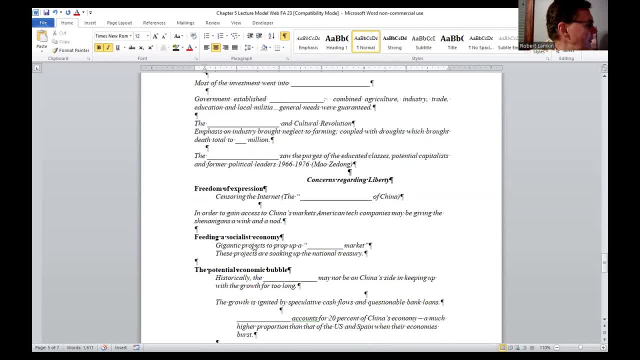 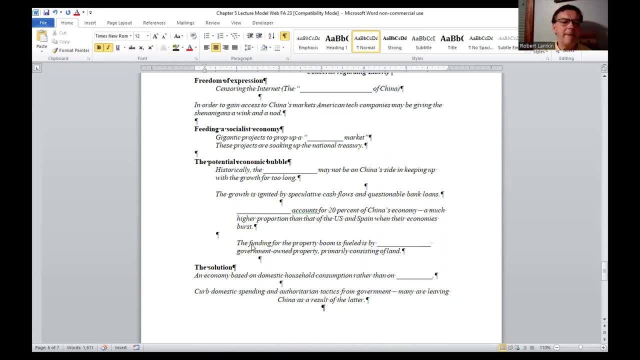 and so you have this potential economic bubble and historically, the law of averages are not on China's side in keeping up with all that growth I talked about not for too long. because here's the thing: some of the cancers I guess underneath the growth is ignited by 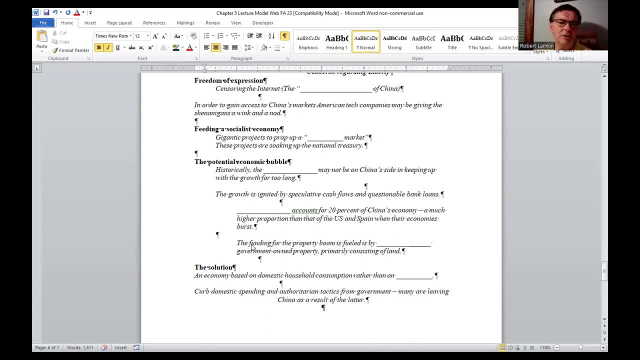 speculative cash flows and questionable bank loans. pardon me, let me turn this off: speculative cash flows and questionable bank loans. real estate accounts for 20% of China's economy, a much higher proportion than that of the United States and Spain when their economies burst. the funding for the property 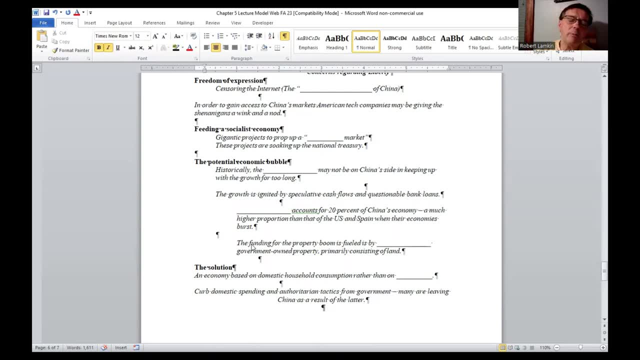 boom is fueled by the overvalued government owned property, primarily consisting of land. So the solution, the way I see it, is an economy based on, maybe, household consumption rather than on exports. So you'll want to curb domestic spending and authoritarian tactics rather than you know from government. 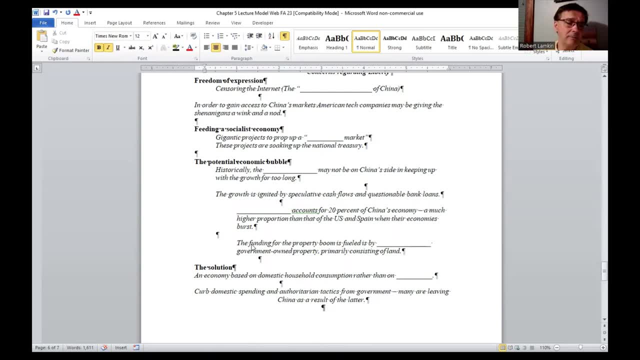 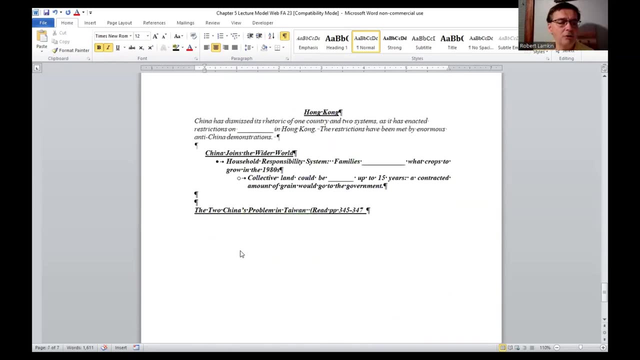 as many are leaving China as a result Of the latter. Then you got the problem of Hong Kong right. You got the problem of Hong Kong. China has dismissed its rhetoric of one country and two systems, as it has enacted restrictions of freedom in Hong Kong. 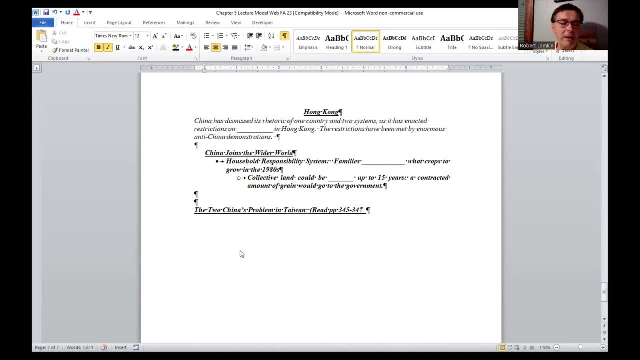 The restrictions have been met by enormous anti-China demonstrations. unfortunately, um we- you know, the current administration- has been uh really silent about this. uh the um again. uh, people in high places in the athletic world have been uh silent about it as well. so hong kong, the british colony right for 100 years and the brits gave that back um. 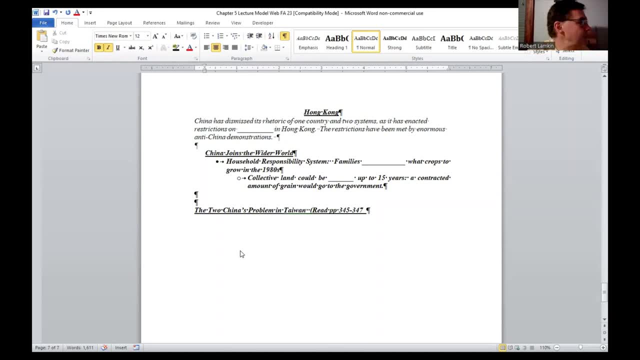 in 1997. so lastly, um china's two problem: china or china's problem in taiwan. i want you to read, uh, pages 345 to 347, and uh, you will be responsible for knowing that, because that information will show up on the quiz as uh as well. okay, so let's um.